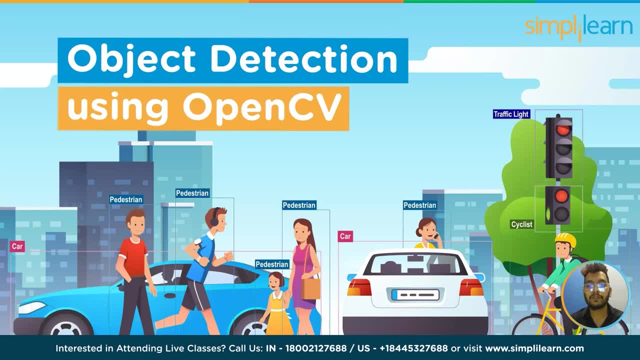 significant improvement. Hello everyone, I am Mayank and welcome to Simply Learn. Today, we will take you through a hands-on live demo of how to do object detection using OpenCV. For amazing videos like this, subscribe to our YouTube channel and press the bell icon. 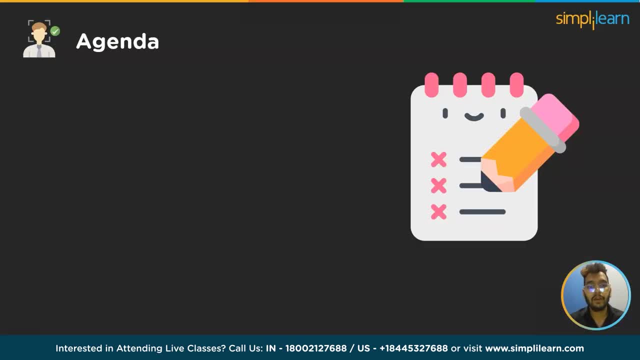 to stay updated. So in today's session we will discuss what OpenCV is and, moving ahead, we will see what is object detection and at the end we will do a hands-on live demo of object detection using OpenCV. In fact, study says there will be more than. 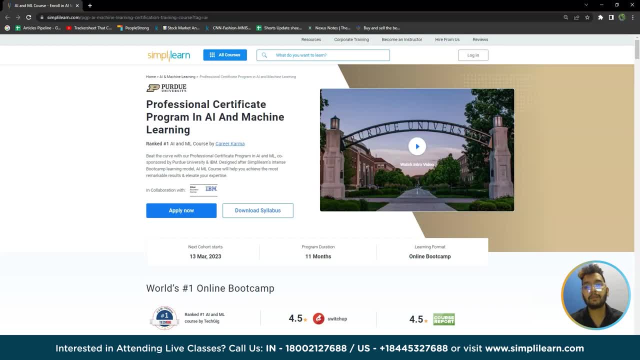 2.3 million job openings in the field of artificial intelligence and machine learning by 2023.. But you can beat the curve with our professional certificate program in AI and machine learning, co-sponsored by Purdue University and IBM, which is designed after Simply Learn's intense 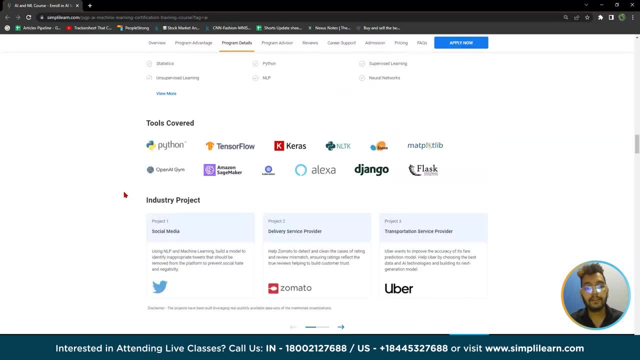 bootcamp learning model AI and ML certification course. This course covers tools and techniques like Python, TensorFlow, Keras, NLTK and many more, along with industry projects like social media by Twitter delivery service provider by Zomato transportation services. 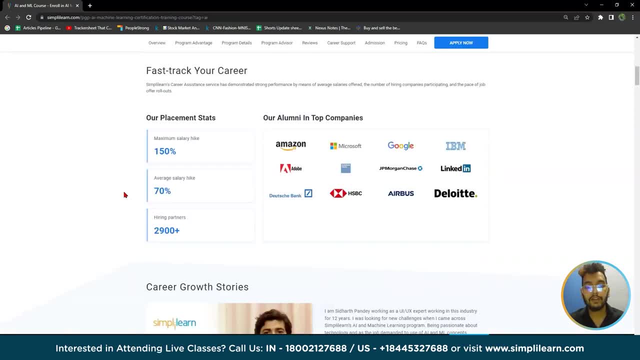 provider by Uber and many more amazing projects. So, choosing this course, you can get hired on renowned companies like Google, Amazon, LinkedIn and Adobe and an average salary hike of 70%. So what are you waiting for? Join the AI and ML certificate program and 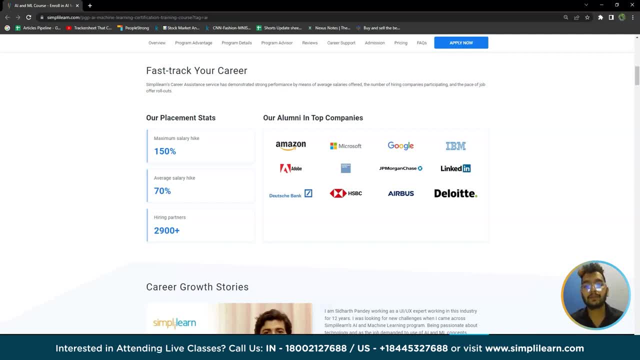 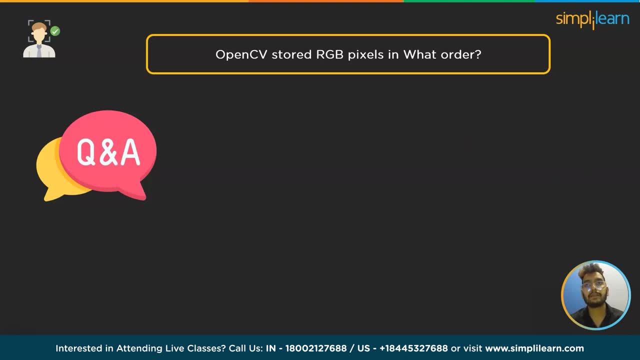 excel your career in artificial intelligence. The link is in the description box below. Before starting, let us have a simple question to brush up your knowledge. So OpenCV stored RGB pixels in what order? GBR, RGB, BGR and RGB. 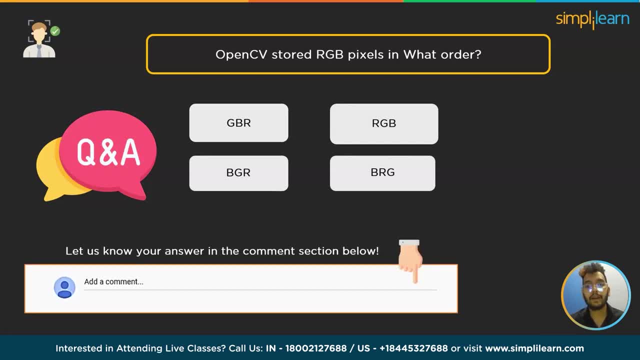 Please answer in the comment section below and we will update the current answer in the pinned comment, Or you can pause the video, give it a thought and answer in the comment section. Before we move on to the programming part, let's discuss what OpenCV is and proceed further. 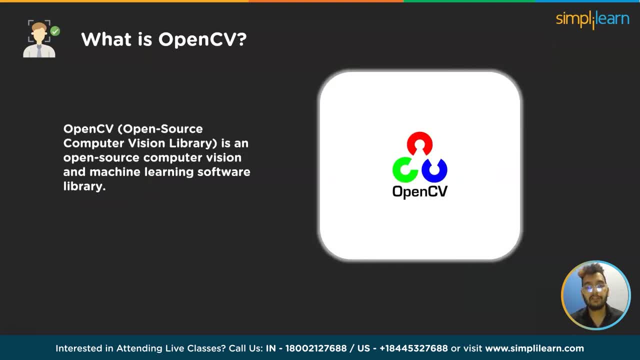 for the same. OpenCV, Open Source Computer Vision Library, is an open source computer vision and machine learning software library. It is written in C++, but has a binding for various programming languages such as Python, Java and MATLAB. OpenCV is an open source computer vision and machine learning software library. It is written 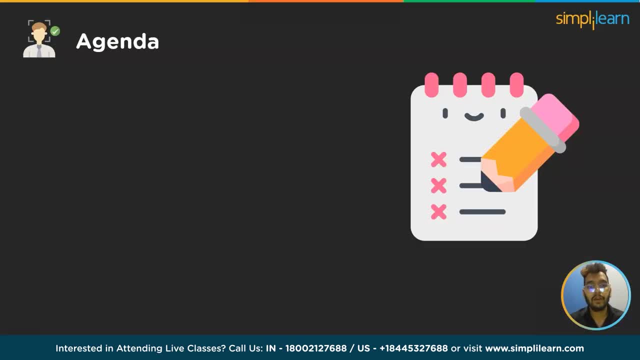 to stay updated. So in today's session we will discuss what OpenCV is and, moving ahead, we will see what is object detection and at the end we will do a hands-on live demo of object detection using OpenCV. In fact, study says there will be more than. 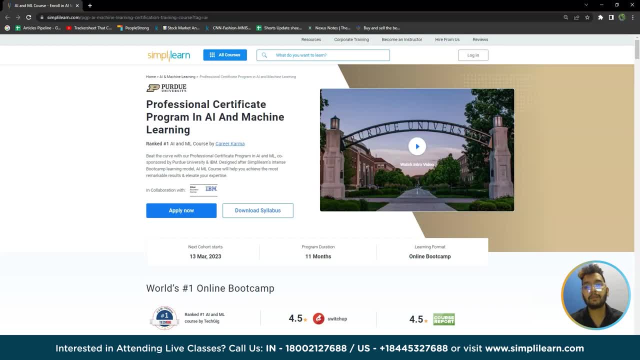 2.3 million job openings in the field of artificial intelligence and machine learning by 2023.. But you can beat the curve with our professional certificate program in AI and machine learning, co-sponsored by Purdue University and IBM, which is designed after Simply Learn's intense 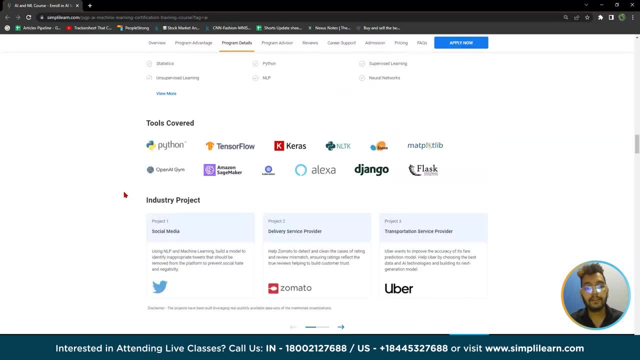 bootcamp learning model: AI and ML certification course. This course covers tools and techniques like Python, TensorFlow, Keras, NLTK and many more, along with industry projects like Social Media. by Twitter Delivery Service Provider. by Zomato Transportation Service Provider. 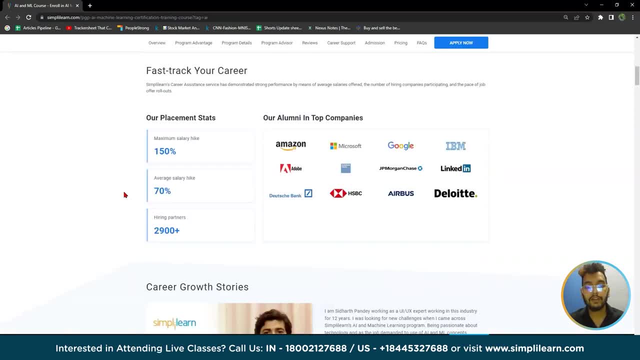 by Uber and many more amazing projects. So, choosing this course, you can get hired on renowned companies like Google, Amazon, LinkedIn and Adobe and an average salary hike of 70%. So what are you waiting for? Join the AI and ML certificate program and 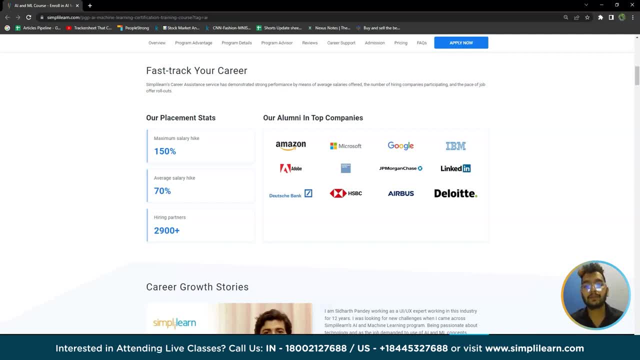 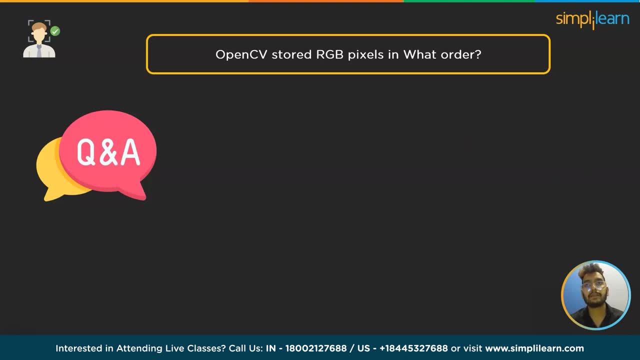 excel your career in artificial intelligence. The link is in the description box below. Before starting, let us have a simple question to brush up your knowledge. So OpenCV stored RGB pixels in what order? GBR, RGB, BGR and RGB. 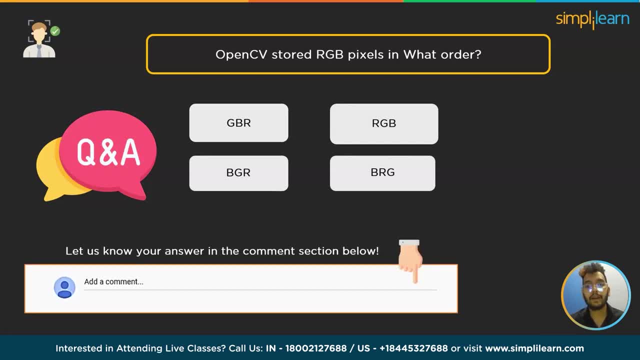 Please answer in the comment section below and we will update the current answer in the pinned comment, Or you can pause the video, give it a thought and answer in the comment section. Before we move on to the programming part, let's discuss what OpenCV is and proceed further. 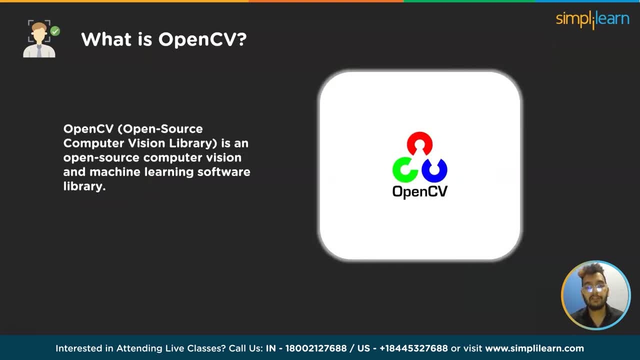 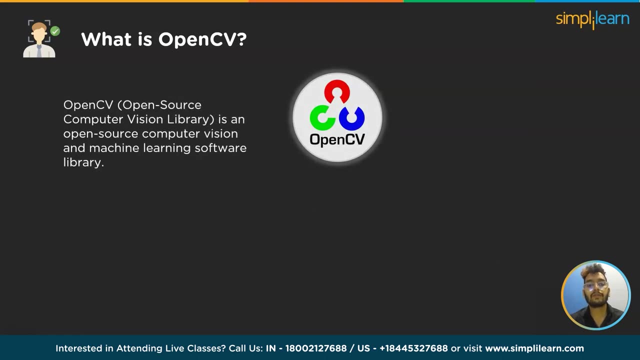 for the same. OpenCV. Open Source Computer Vision Library is an open source computer vision and machine learning software library. It is written in C++ but has a binding for various programming languages such as Python, Java and MATLAB. OpenCV was designed with the goal of providing a common infrastructure for computer vision. 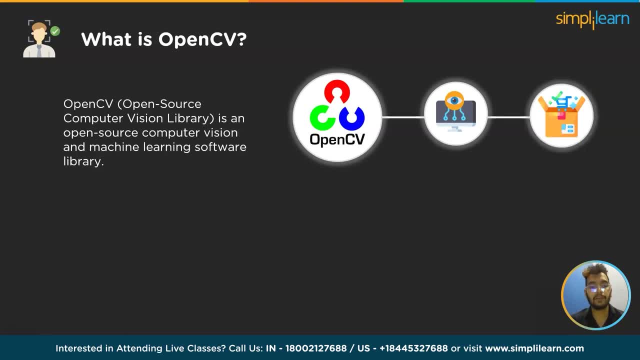 applications and to accelerate the use of machine learning perception in a commercial product widely used in a variety of industries, including robotics, automotive and healthcare. It's supported by a large community of developers, researchers and users who contribute to its development and provide support to its users. 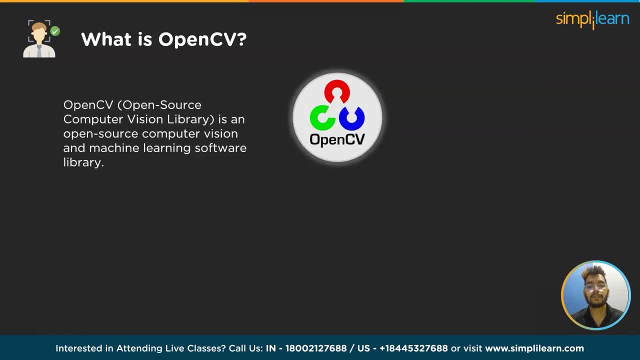 in C++ but has a binding for various programming languages such as Python, Java, MATLAB. OpenCV was designed with the goal of providing a common infrastructure for computer vision applications and to accelerate the use of machine learning perception in commercial products. OpenCV is widely used in a variety of industries, including robotics, automotive and healthcare. 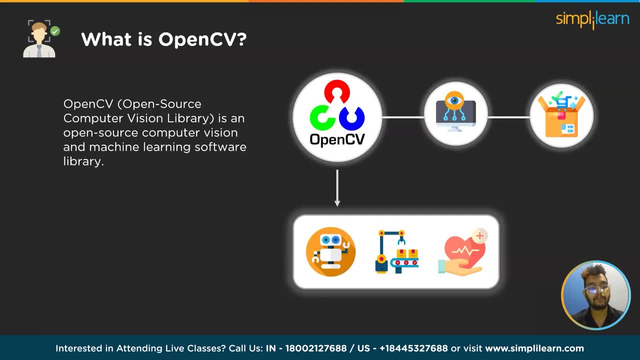 It is supported by a large community of developers, researchers and users who contribute to its development and provide support to its users. It is supported by a large community of developers, researchers and users who contribute to its development and provide support to its users. 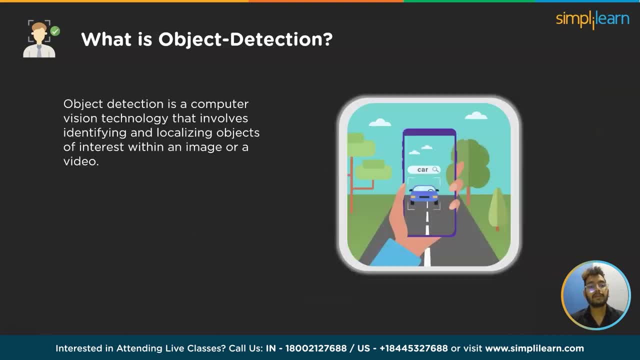 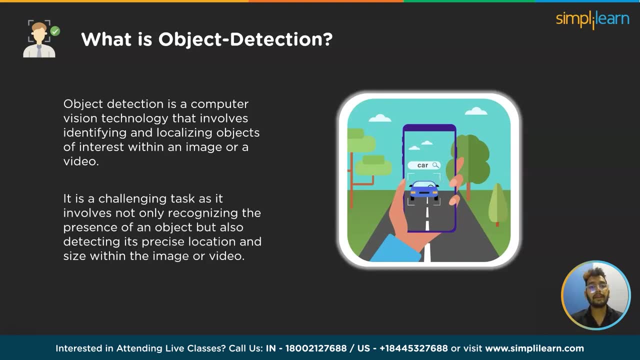 users. Now let's see what is object detection. Object detection is a computer vision technology that involves identifying and localizing the object of interest within an image or a video. It is a challenging task, as it involves not only recognizing the presence of an object. 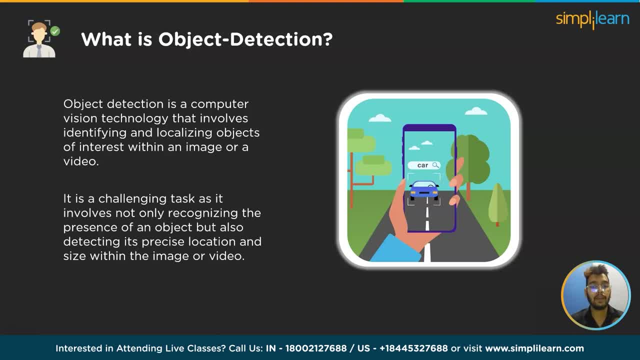 but also detecting its precise location and size within the image or video. Object detection algorithm typically used deep learning techniques, such as CNN, to analyze the image or video for identifying the objects. These algorithms can also determine the boundaries of the object by drawing a bounding box around them. So, after understanding what is object detection, 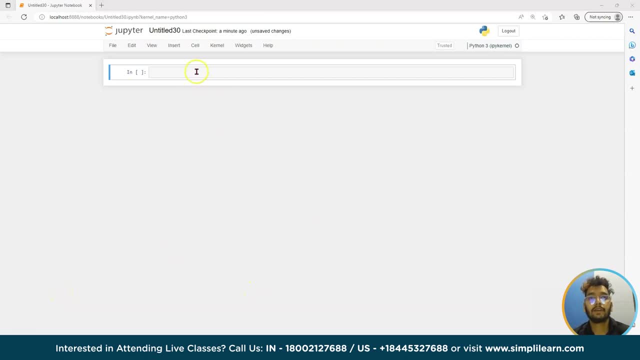 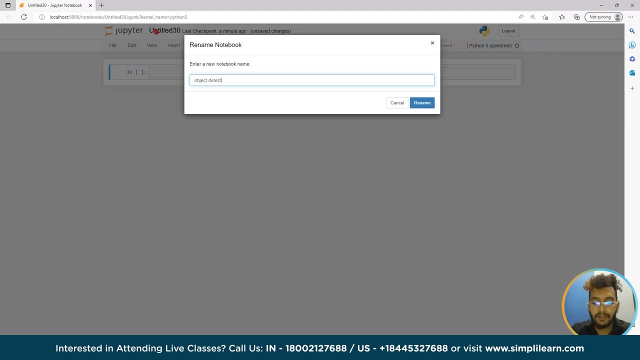 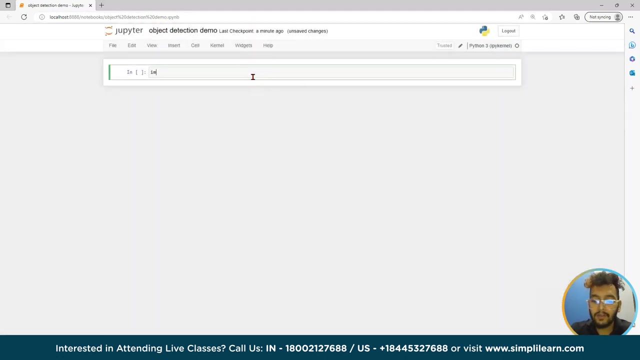 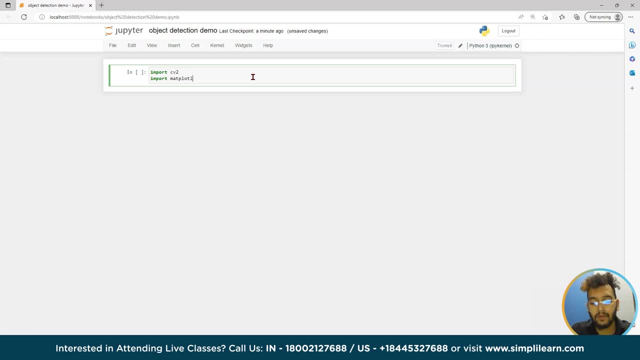 import matplotlibpyplot as plt. So why we are writing plt? because we can't write again and again matplotlibpyplot. Okay, it's a long one, so we can write a short form plt. So yeah, let's run this. So what is opencv? Opencv is an open source software library. 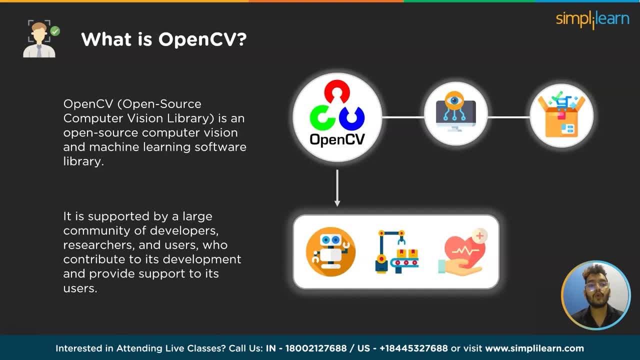 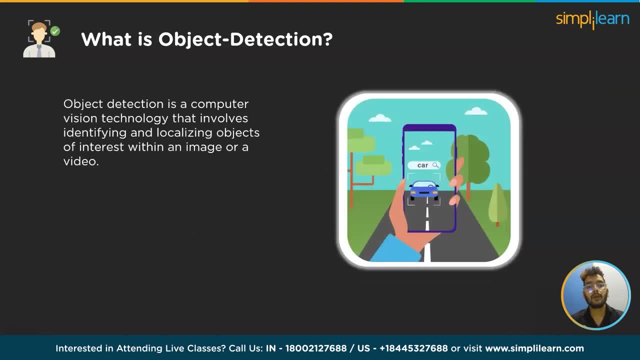 It is supported by a large community of developers, researchers and users who contribute to its development and provide support to its users. Now let's see what is object detection. Object detection is a computer vision technology that involves identifying and localizing the object of interest within an image or a video. 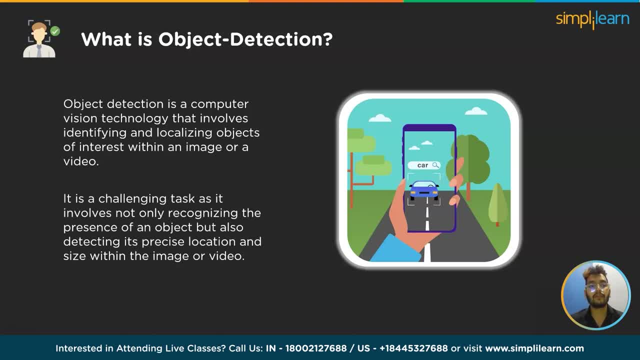 It is a challenging task, as it involves not only recognizing the presence of an object, but also detecting its precise location and size within the image or video. Object detection algorithms typically use deep learning techniques, such as CNN, to analyze the image or video for identifying the objects. 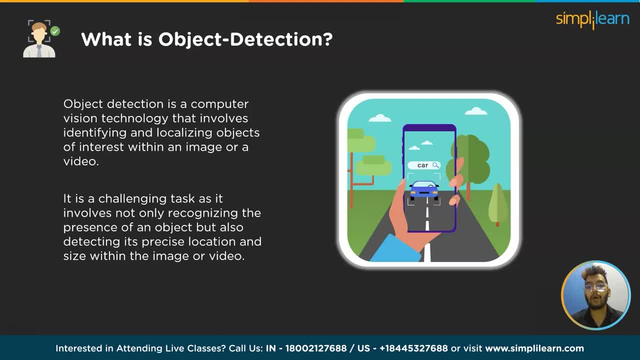 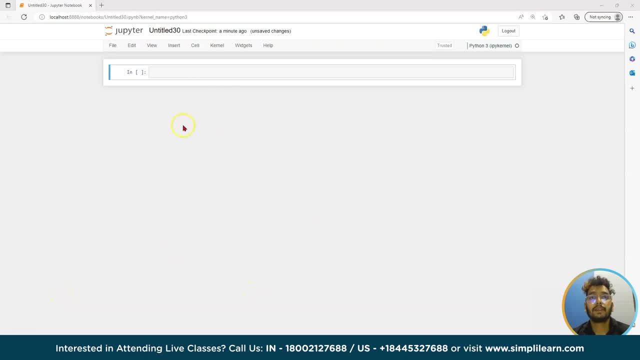 These algorithms can also determine the boundaries of the object by drawing a bounding box around them. So after understanding what is object detection, now let's move on to the programming part. This is a computer vision. We have a Python kernel Here. we will change this name. 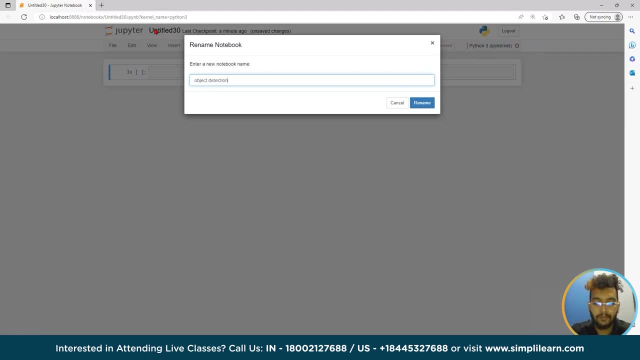 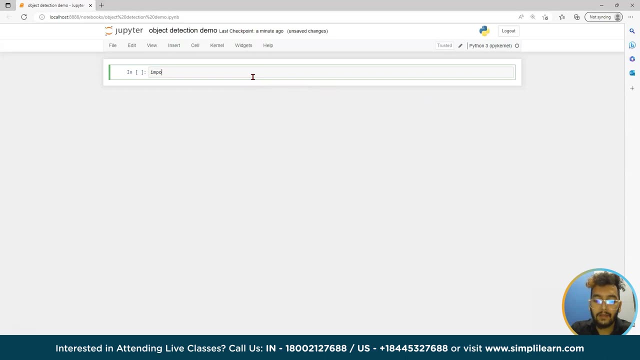 So here I will write object detection demo. First we will import some major library like OpenCV, So for that we will write import cv2, and the next one is import matplotlibpyplot. So why we are writing plt? because we can't write again and again matplotlibpyplot. 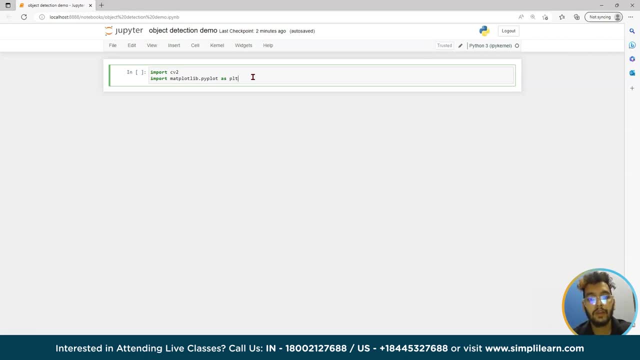 Okay, it's a long one, so we can write a short form plt. So yeah, let's run this. So what is OpenCV? OpenCV is an open source software library for computer vision and machine learning. The OpenCV full form is open source computer vision library. 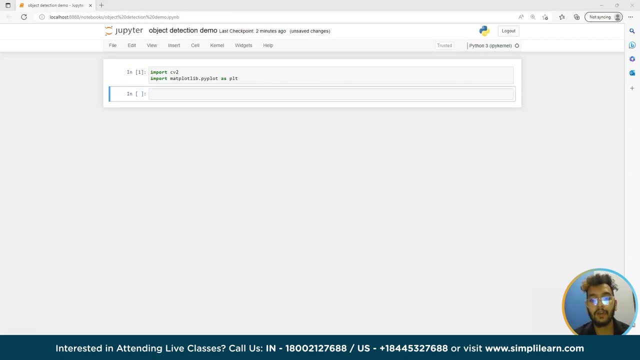 It was created to provide a shared infrastructure for application for computer vision and to speed up the use of computer vision. The OpenCV has a BSD license software. make it simple for companies to use and change the code. Okay, so there are some predefined packages and libraries that make our life simple and 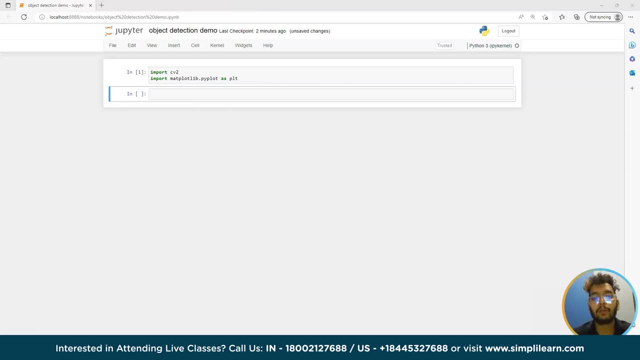 OpenCV is one of them. Again, one is matplotlib. matplotlib is an easy to use and an amazing visualized library in Python. It is built on NumPy array and designed to work with broader scipy stack, and consists of several plots like line bar, scatter, histogram. 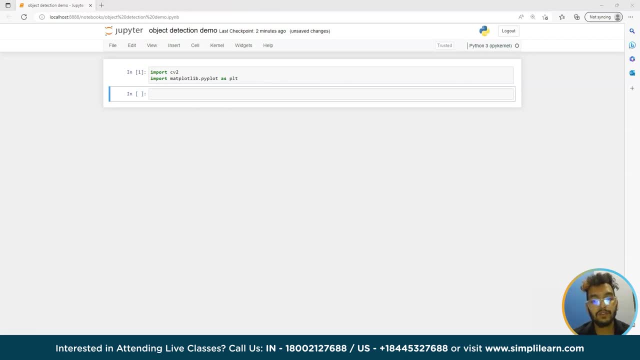 for computer vision and machine learning. The opencv full form is a open source computer vision library. it was created to provide a shared infrastructure for application for computer vision and to speed up the use of machine learning perception in consumer products. opencv, as a bsd license software, make it simple for companies to use and change the code. okay, so. 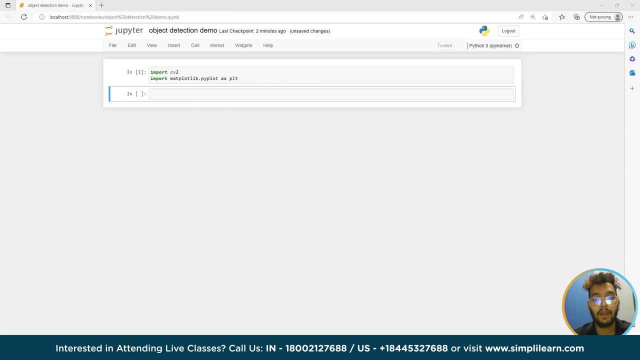 there are some predefined packages and libraries that make our life simple, and opencv is one of them. second one is matplotlib. matplotlib is a easy to use and an amazing visualize library in python. it is built on numpy array and designed to work with broader scipy stack, and consists of several. 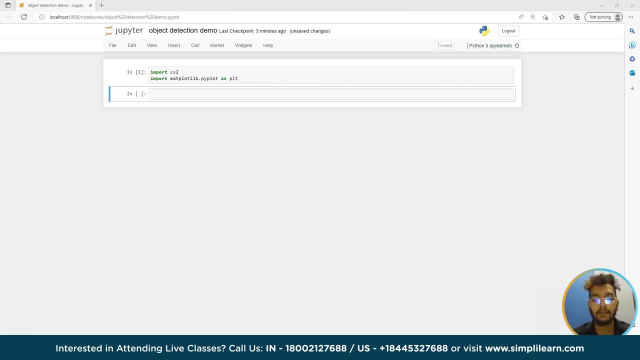 plots like line bar, scatter, histogram and many others. okay, so, moving forward, we will import our file. okay, so here i will write. config. file goes to: this is our file name: ssd. underscore mobile net. so v3 large coco 22, contain dot bb. okay, so you can find this file on the description box below. 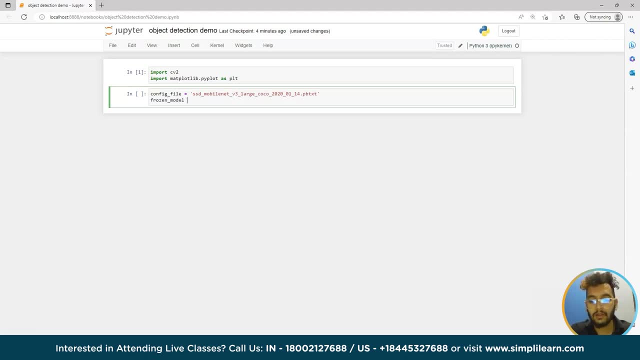 frozen model question. so i will explain you every single thing. inference graph- dot pb. okay, so let me run it first. mobile net as a name applied. the mobile net model is designed to use in mobile application and it's tensorflow first mobile computer vision model. mobile net use depthwise separable convolutions. it significantly reduces the numbers of parameter. 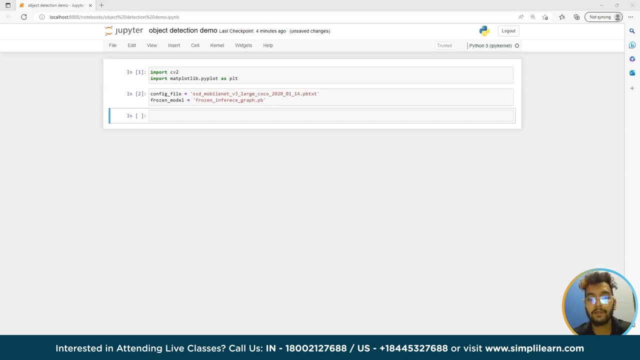 when compared to the network with regular convolutions with the same number of parameters depth in their eggs, this is in the lightweight of the deep neural network. so mobile net is a glass of cnn that was open source by google and therefore this gives us an excellent starting point for training our classifiers that are insanely small. 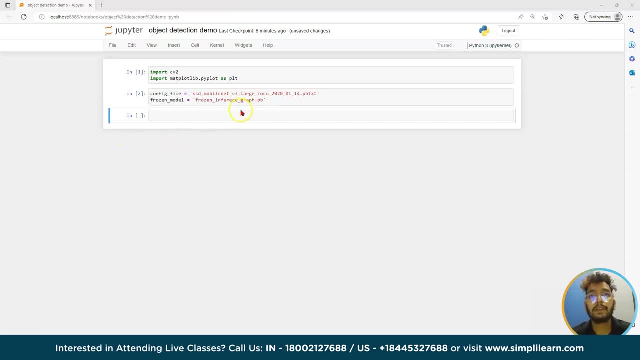 and insanely fast. okay, so what is this large coco? this is a dataset coco dataset. like with applications such as object detection, segmentation and captioning, the coco data set is widely understood by the state of the art of neural network. its versatility and results in speciality are more reflected, etc. looking at the concept of copostat tree, use it like a string. this one is a. 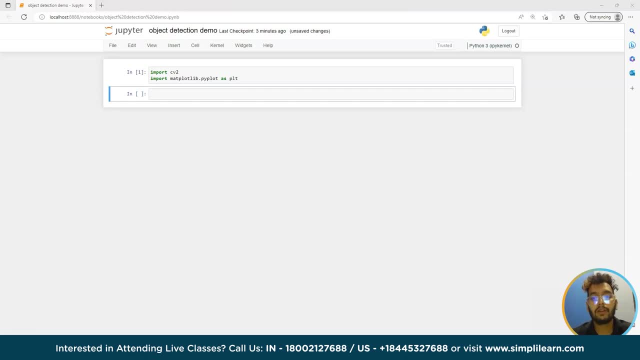 And many others. Okay so, moving forward, we will import our file. Okay so here I will write. config file goes to: this is our file name: SSD underscore mobile net v3, large, coco 22.. Okay so you can find this file on the description box below: frozen model question. 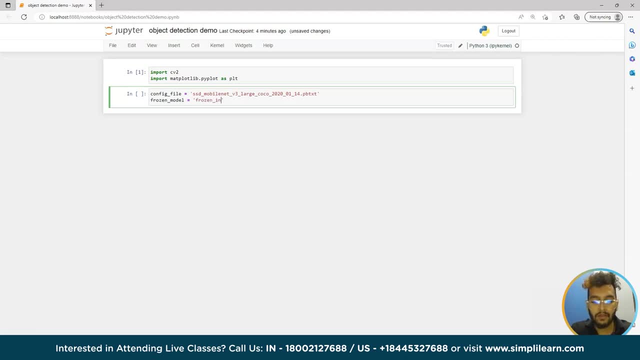 I will explain you every single thing. Inference Graph dot bb. Okay, So let me run it first. mobile net As a name applied. the mobile net model is designed to use in mobile application and it's TensorFlow first mobile computer vision model. mobile net use depthwise separable convolutions. 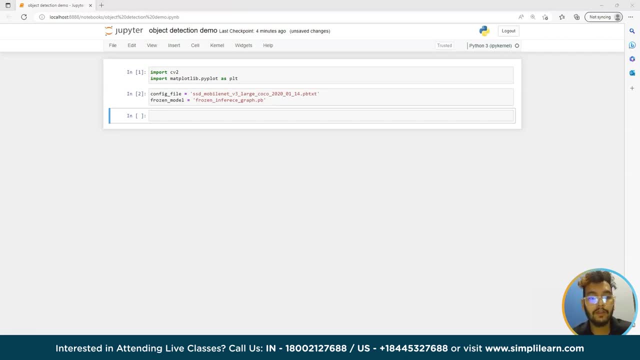 It significantly reduces the numbers of parameter when compared to the network with regular convolutions with the same depth in the nets. This is that in the lightweight of the deep neural network. So mobile net is a class of CNN that was open source by Google. 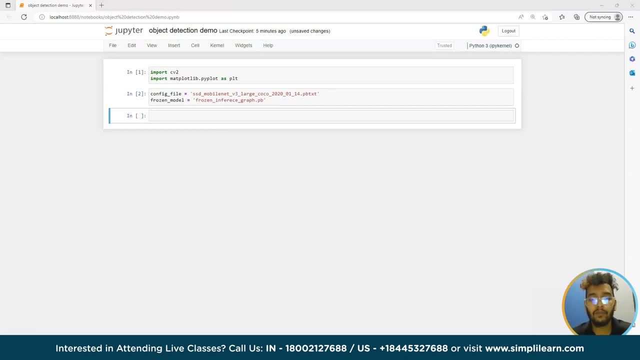 And therefore this gives us an excellent starting point for training our classifiers that are insanely small and insanely fast. Okay, so what is this large coco? This is a data set- coco data set, like with applications such as object detection, segmentation and captioning. 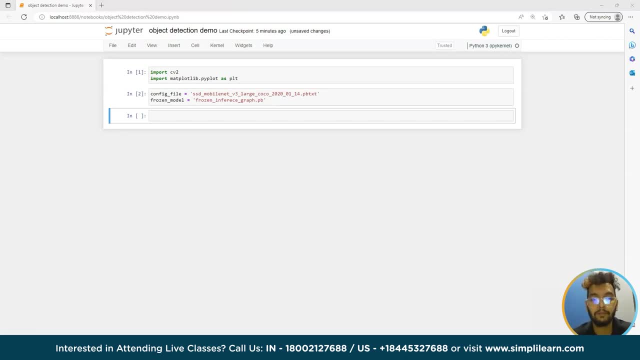 The coco data set is widely understood by the state of the art of neural network. It's versatility and the multipurpose scene variations are best to train a computer vision model and benchmark its performance. Okay, so what is coco? Okay, The common object in context is one of the most popular large scale label images, data. 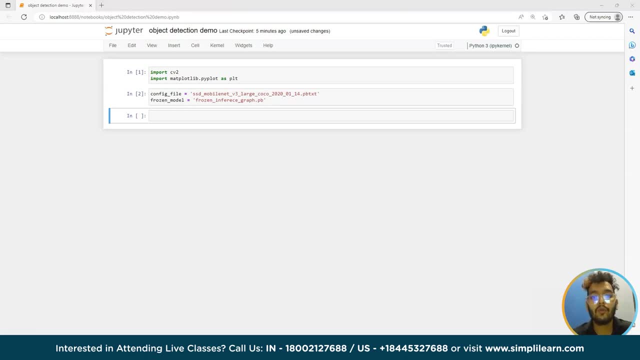 set available for public use. It represents a handful of objects we encounter on a daily basis and contains image annotations in 80 categories. I will show you the categories I have with over 1.5 million object instances. Okay, so modern day AI driven solution are still not capable of producing absolute accuracy. 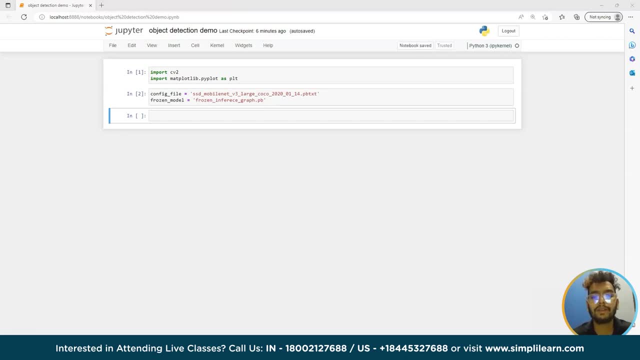 in result, which comes down to the fact that coco data set is a major benchmark for the modern day AI driven solution. The coco data set is a supplement to transfer learning, where the data used for one model serves as a starting point for the another. large coco. its versatility isn't a big challenge to bb user. okay, собой, that means you will be viewing this video. i will show you how you can contributes to this. uh, for the need, the Hardtex or global où. you could do it like these channels or other things. but i will show you some other possibilities and which are attractive, dynamic, of web purposes. 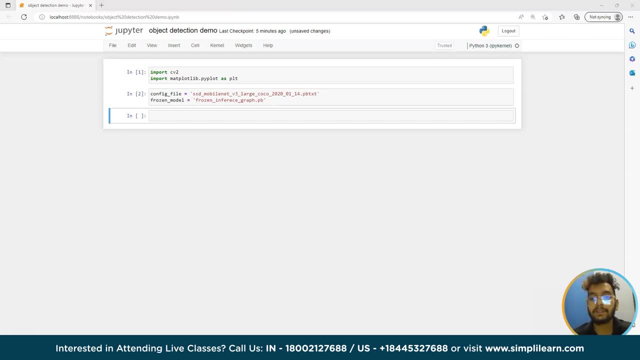 its versatility and the multi-purpose scene variation serve best to train a computer vision model and benchmark its performance. okay, so what is coco? the common object in context is one of the most popular large-scale labeled images data set available for public use. it represent a handful of object we encounter on a daily basis and contains image annotations in 80 categories. i 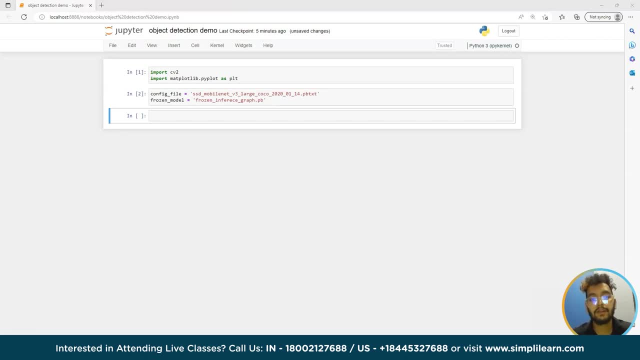 will show you the categories i have with over 1.5 million object instances. okay, so modern day ai driven solution are still not capable of producing absolute accuracy and result, which comes down to the fact that coco data set is a major benchmark for cv to train, test and polish refined models. 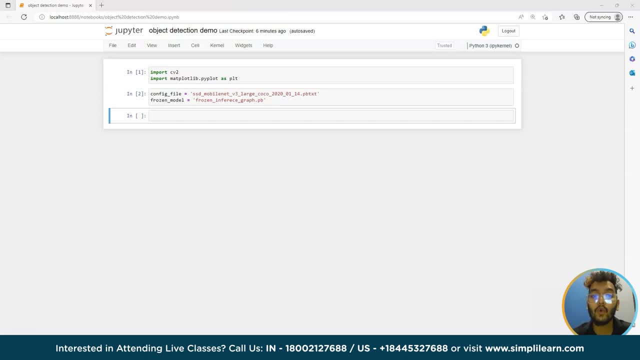 for faster scaling of the annotation pipeline. on the top of that, the coco data set is a supplement to transfer learning, where the data used for one model serves as a starting point for the another. so what is frozen instance graph like? freezing is the process to identify and save all the required graphs, like 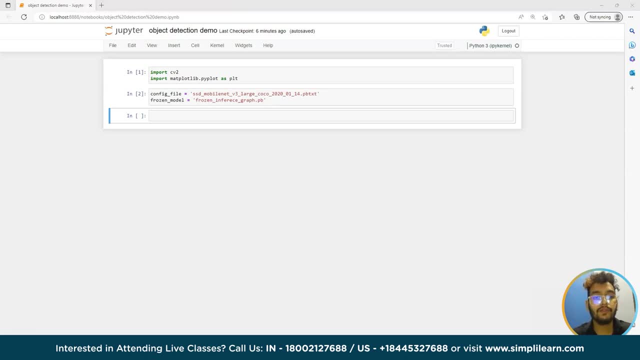 weights and many others in a single file that you can usually use. a typical transfer flow model contains four files and this contains a complete graph. okay, so forward, let's create one model here. i will write model first to cv2, dot dnn model and then i will use barni's gdn index, the большое number feature that we used for some gdn index. 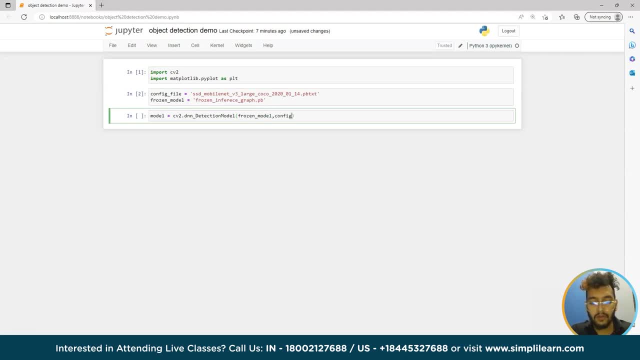 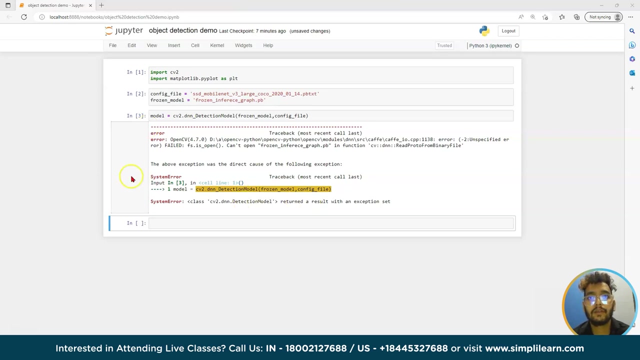 those values we can put right. dash was done. and then config file. so here i am giving the parameters, two parameters like frozen model and config file. we go over here. you run it first. okay, there is error return. ok, so cv2 dot dn and direction model return is: 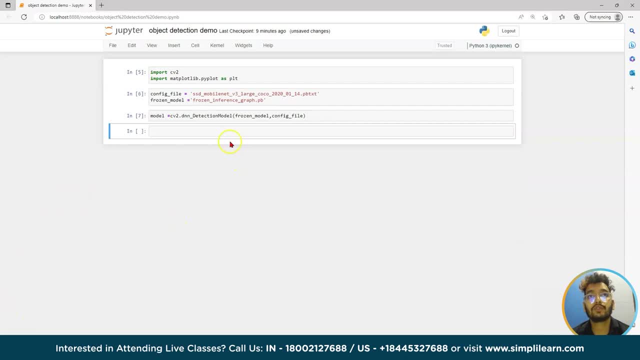 and then exception set. then the Seo in this scenario is from the htirotion which i will give in another comment. The question comes: what is the meaning of detection model or DNN detection model? This class represents the high-level API for object detection networks. 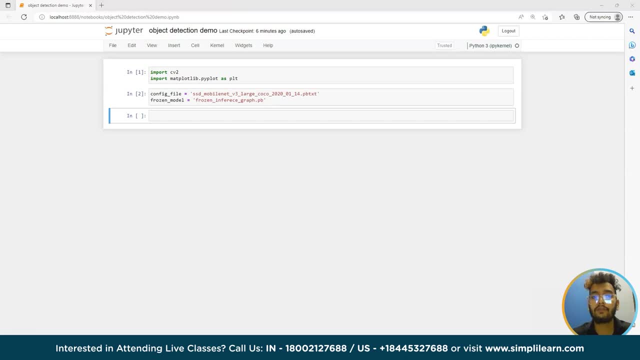 So what is frozen inference graph? Like freezing is the process to identify and save all the required graphs, like weights and many others, in a single file that you can usually use. A typical transfer flow model contains four files and this contains a complete graph. Okay, 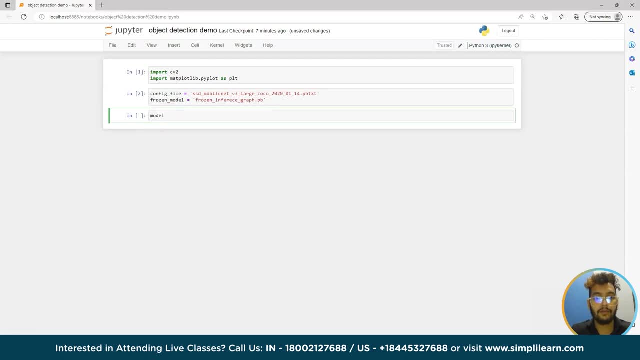 So how about let's create one model that I will write, model first to cv2.dnn, model frozen and then config file. here I'm giving the parameters, two parameters like frozen model and config file. score. here You run it first. 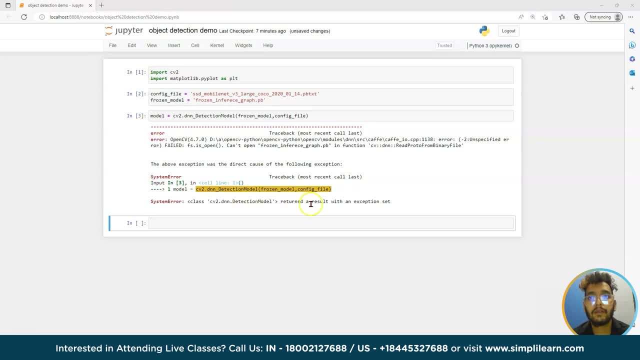 Okay, There is error. you turn the okay. So error is cv2.dnn detection model returned. as result, An exception set. The question comes: what is the meaning of detection model or DNN detection model? So this class represent the high level API for object detection networks. 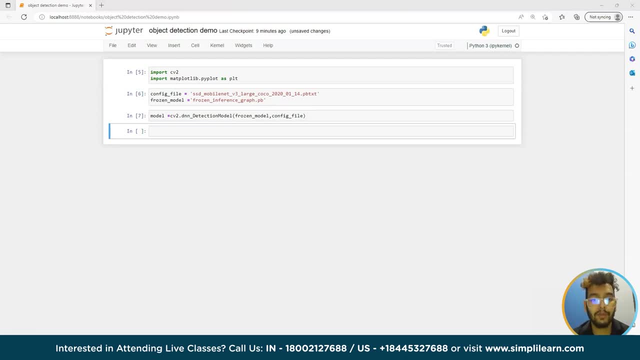 Detection models allows to set parameters for pre-processing input. image Detection model creates net from file from file and with trained weights and config sets it. processing input runs forward, pass and return the result. detection- okay, moving forward, let's set the class labels. okay, class labels. 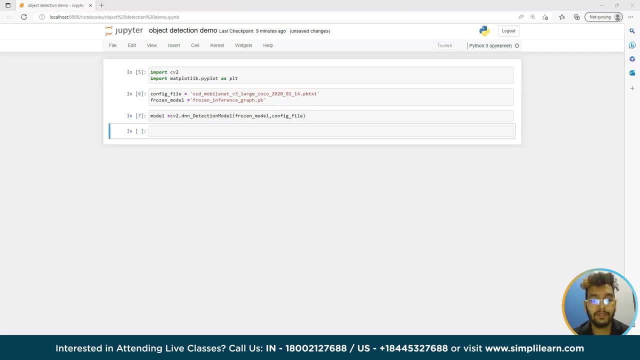 Detection model allows to set parameters for pre-processing input. image Detection model creates net-from file with trained weights and config sets its processing input runs forward pass and returns the result. detection Moving forward, let's set the class labels. class labels, file name, labelstxt. I will 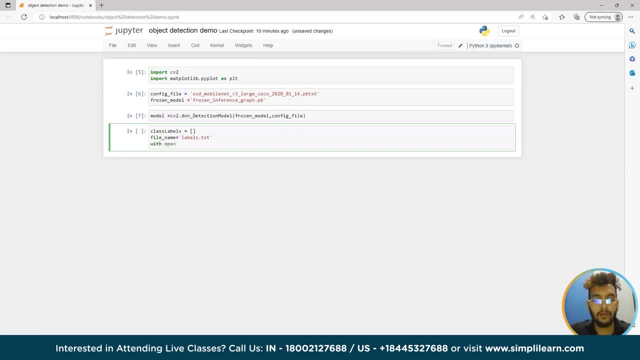 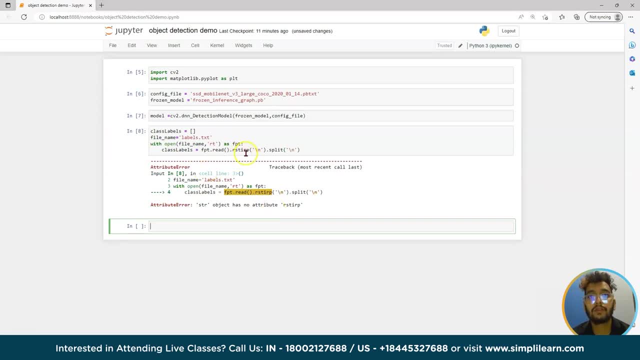 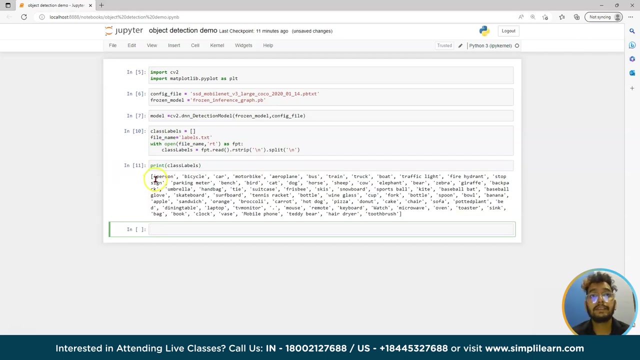 So here I created one array of name, class labels. So this is the file name. What I am doing, I am putting this label file into this class label. Okay, So here, if I will print Now class labels, These are the 80 categories in the cocoa data set. 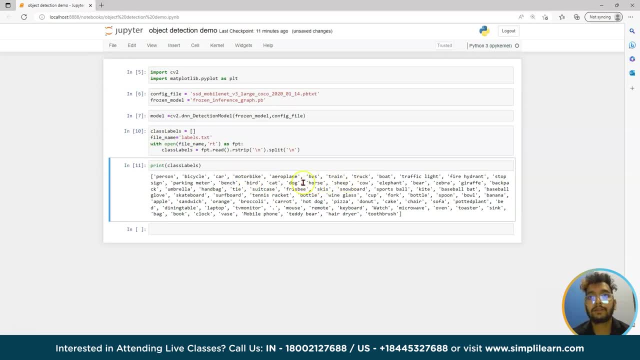 Okay, this person, bicycle, car, motorbike, aeroplane, bus, train. These all are the 80 categories. I Will put this file labeled or txt, in the description box below. you can find download from there. Okay, fine, So let's print the length of the cocoa data set or you can see class labels. 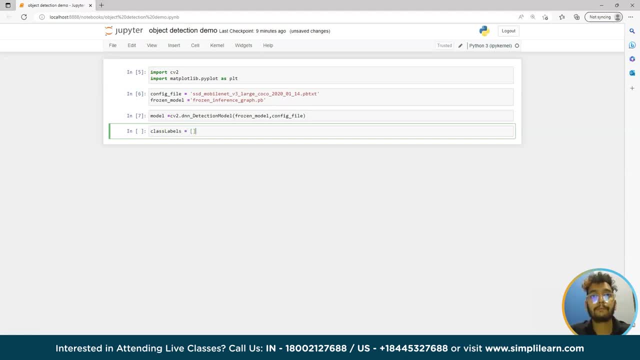 file name, also labelstxt. i will put this file on the description box below. you can download from there. open file name: class labels, history. and So here I created one array of name, class labels. so this is the file name. what I am doing, I am putting this label file into this class label. ok, so here, if I will print class: 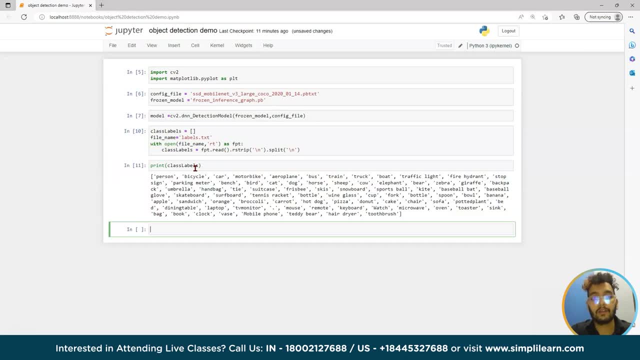 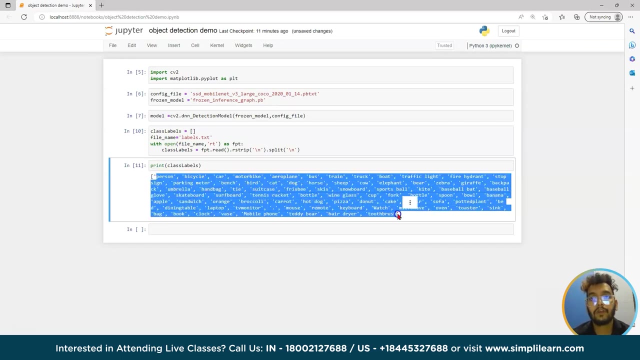 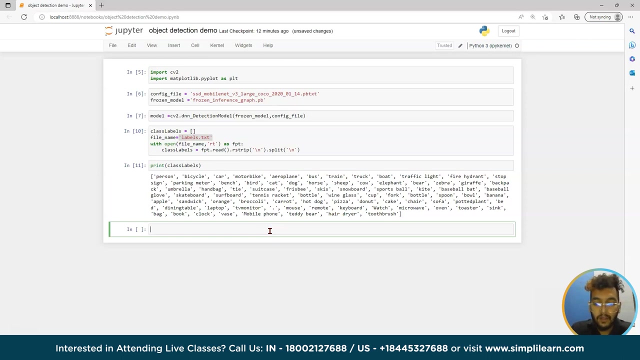 labels. so these are the 80 categories in the coco dataset. ok, this person, bicycle, car, motorbike, aeroplane, bus, train. these all are the 80 categories. I will put this file labeltxt in the description box below. you can download from there. ok, fine, so let's print the length of the coco dataset. 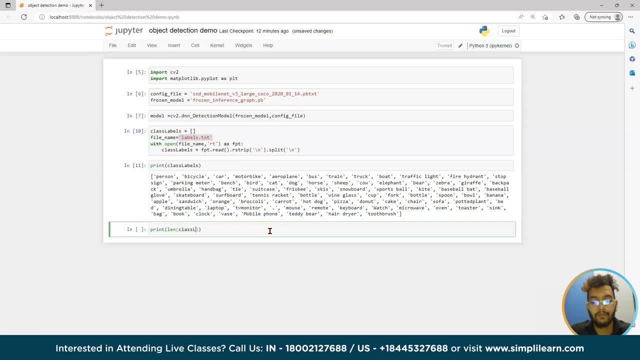 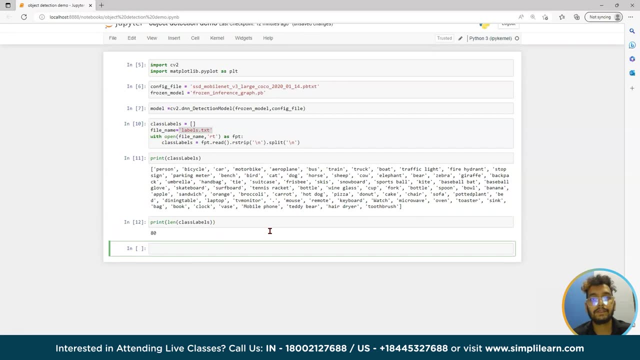 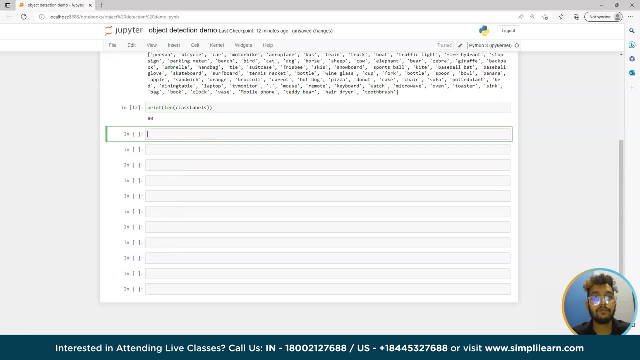 or you can see class labels. this is 80, as you can see. I have already told you the length will be 80, so here let's set this sum: model input size, scaling mean and all. so I will write here: model dot set input size: T20, comma, T20. 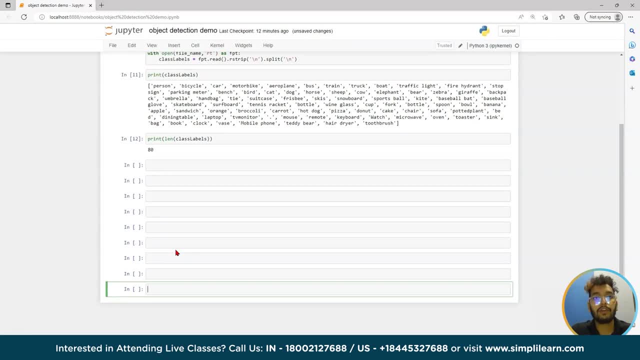 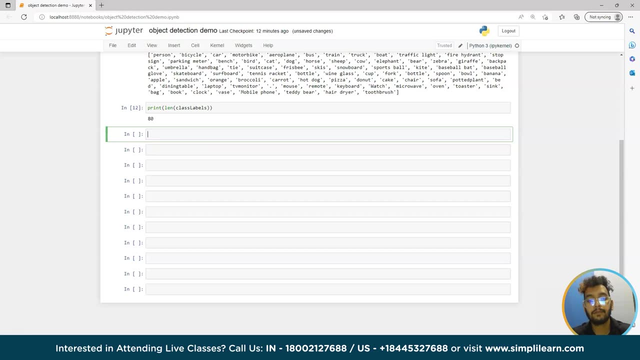 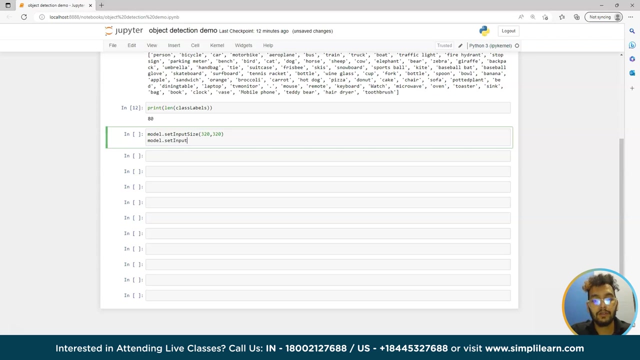 Is 80. as you can see, I have already told you The length will be 80, so here let's Set this some model input size, scaling, mean and all I will write here: model set: what Is 320 Dot set Input Scale 1.0. 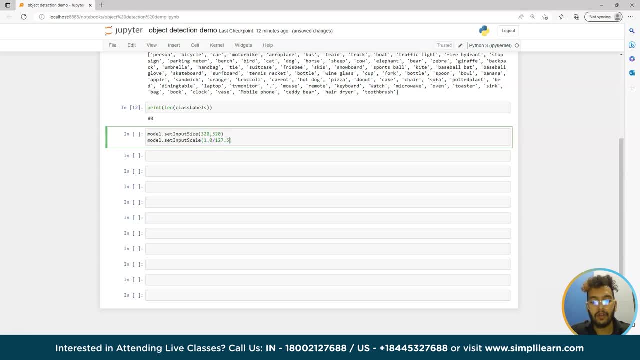 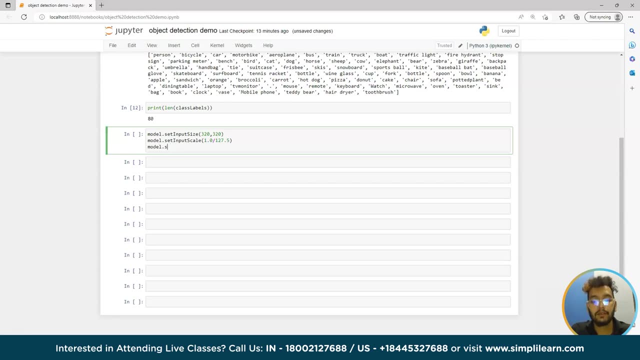 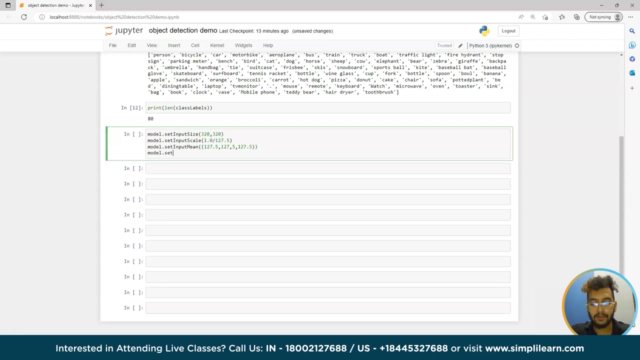 Slash 127, 0.5. Okay, I will explain, you don't worry. model dot set Set: Import me 127, 0.5 comma, 127, 0.5 comma, 127, 0.5. Okay, and then model dot set: What I 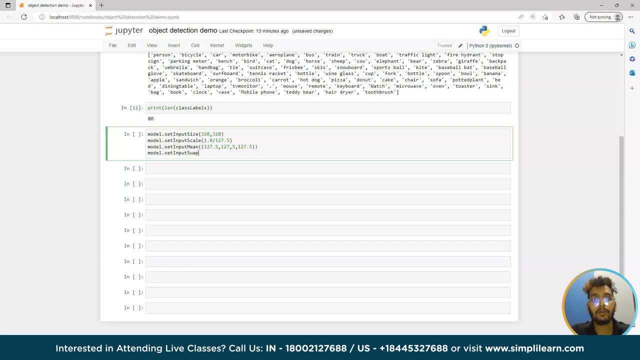 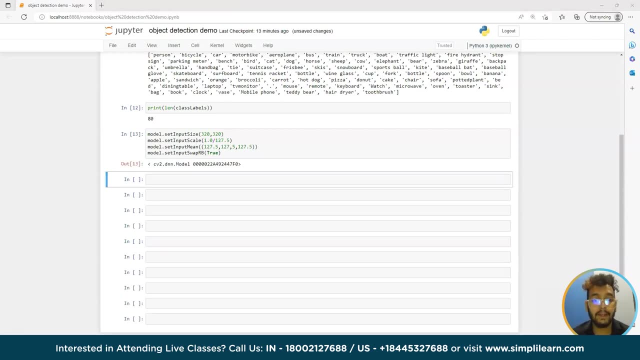 The set input is set input scale. is the set input scale, is the set of the new frame, The shape of the new blob, less than 0? Okay, so this is an size of the new frame. Second, one is set input scale. so set input scale is a scale factor of the value for the frame, or you can say the parameter will. 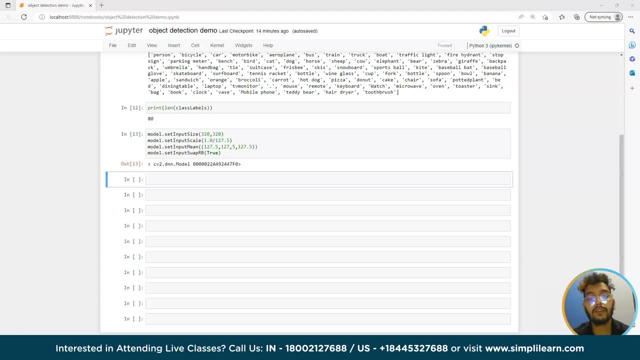 be the multiplier of the frame values, or you can say multiplier for the frame values. okay, so, and input mean so it set the mean value for the frame, the frame in which the photo will come, the video will come or my webcam will come. so it set the mean value for the frame or the for. 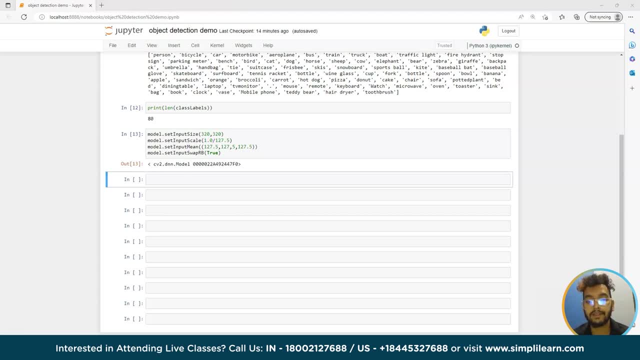 parameters. mean is killer. with the mean values which are subtracted from the channels, you can say: and the last one is set input swap rb. so it set the flag swap rb for the every frame. we don't have to put every time a single frame for a particular image. it will be set the true for. 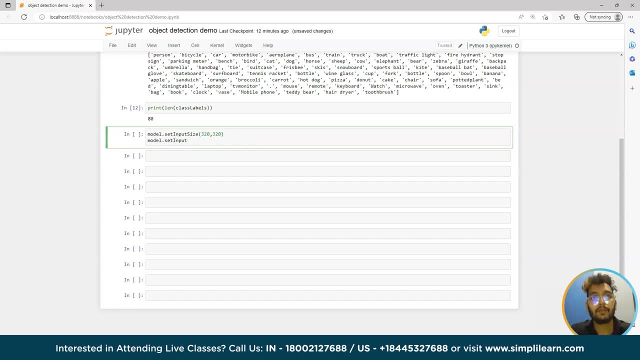 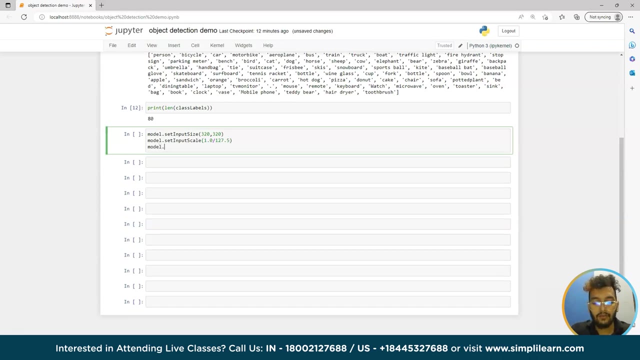 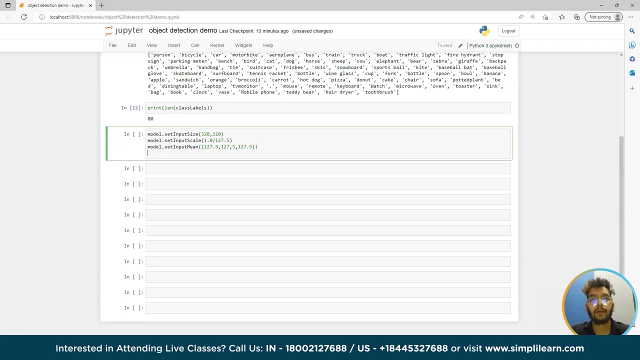 model dot set input scale: 1 point 0, slash 127, point 5: ok, I will explain, you don't worry. model dot set set set set ved set: import me 127.5 comma, 127.5 comma, 127.5. okay, and then model don't set. 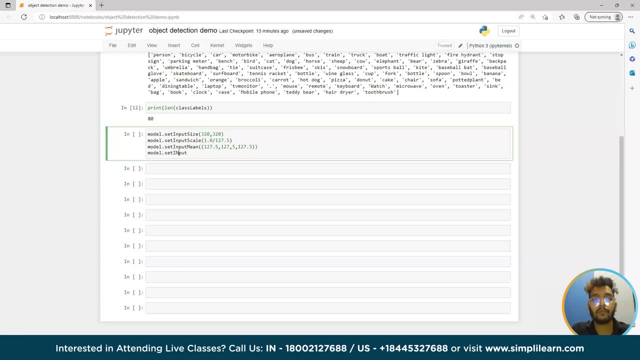 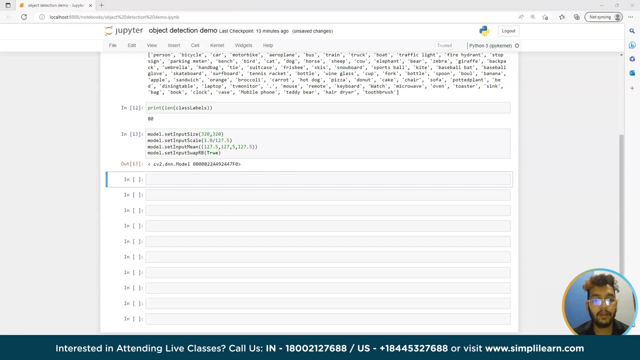 what B? what is set input size? okay, so set input size is a size of new frame, the shape of the new blob, less than zero. okay, so this is the size of the new frame. the second one is set input scale. the set input scale is a scale factor of the value for the frame, or 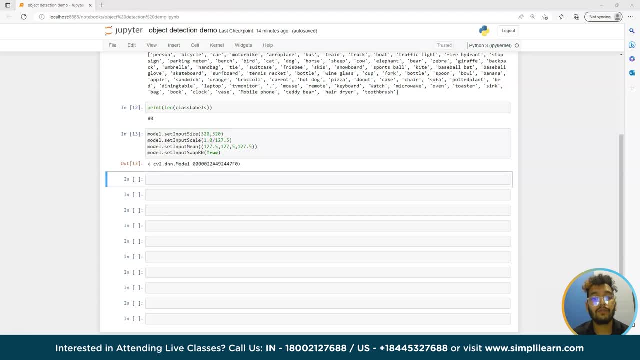 You can say the parameter will be the multiplier of the frame values, or you can say multiplier for the frame values. So input mean. so it set the mean value for the frame, the frame in which the photo will come, the video will come Or my webcam will come. so it set the mean value for the frame or the for parameters. 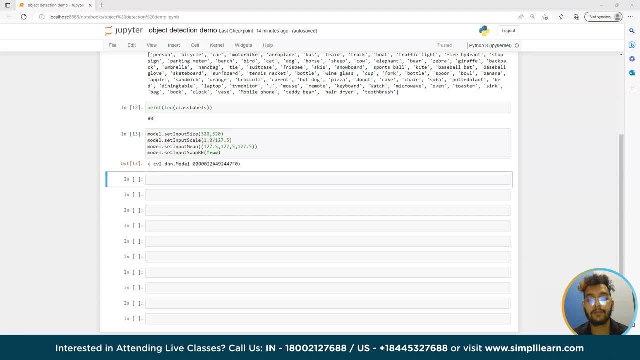 Mean is killer. with the mean values which are subtracted from the channels, you can say: and the last one is set input swap rb. So it's set the flag swap rb for the every frame. We don't have to put every time a single frame for a particular image. 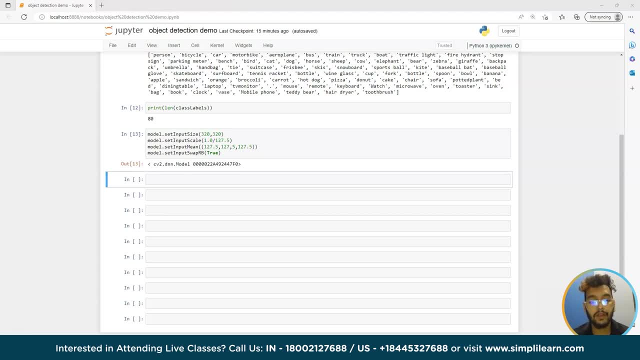 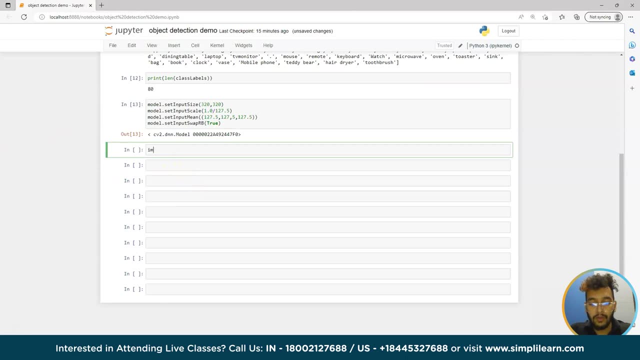 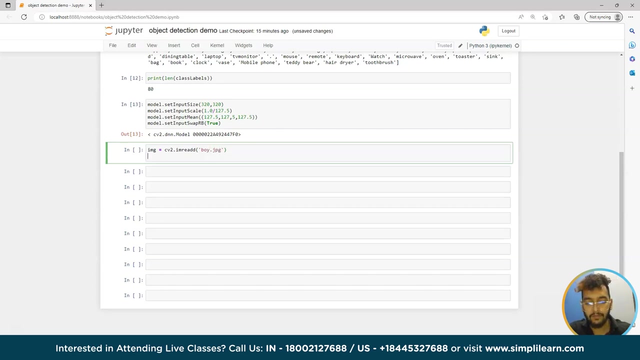 It will be set the true for the all the images. okay, So parameters will be swap rb flag, which indicates a swap first and the last channels. So, moving forward, we will import one image, You, I am read, Boy, don't keep it, Beauty, don't I am sure. 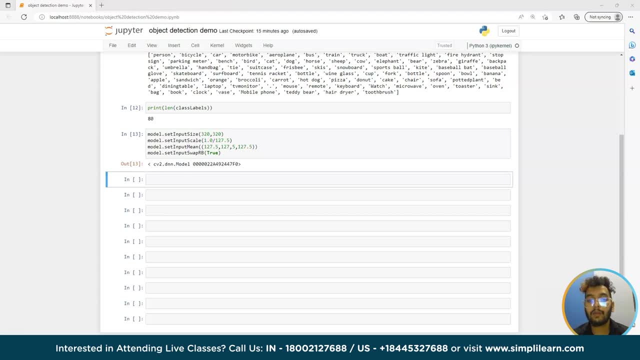 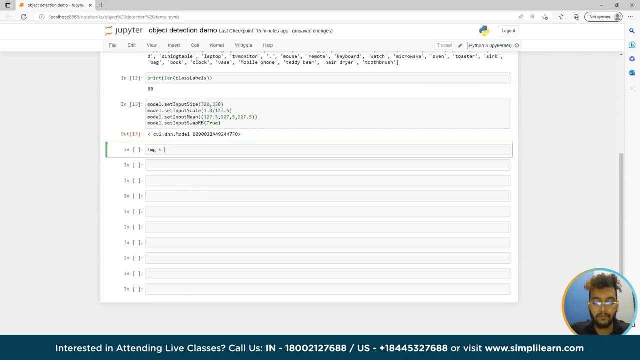 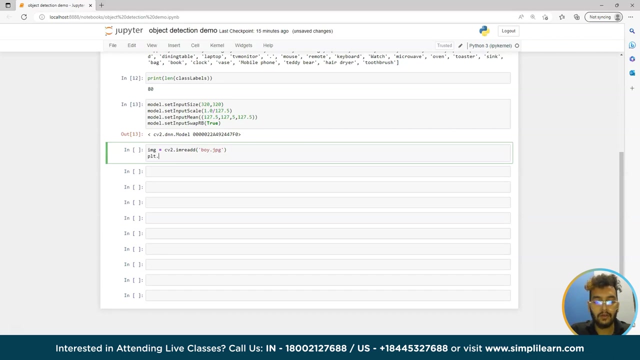 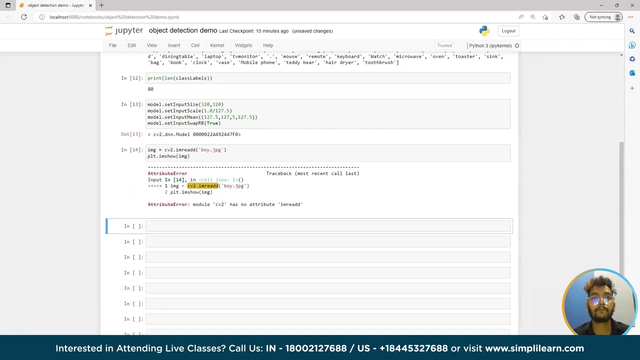 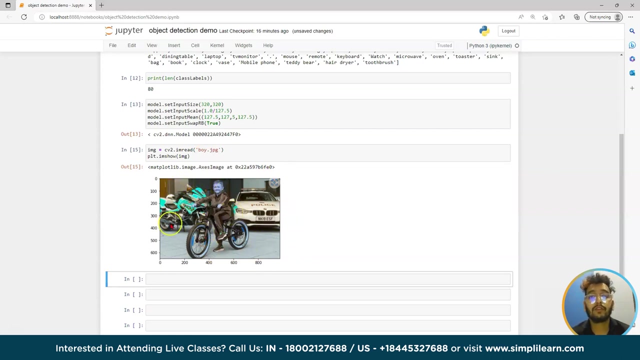 the all the images. okay, so parameters will be swap rb flag, which indicates the swap first and the last channels. so, moving forward, we will import one image. i am read you, I am sure. so this is the size of 320 by 320. okay, so first thing is you can download this, the random. 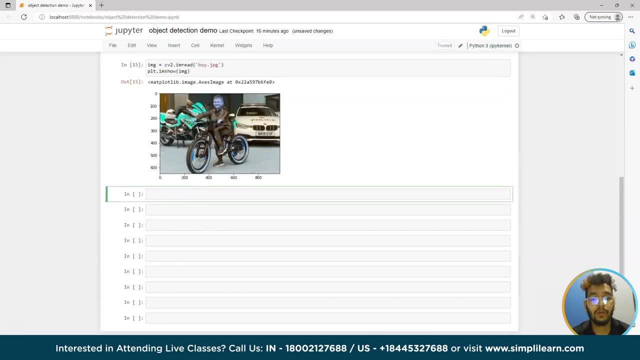 measure from the Google. I took from Google itself. so now what we will do. we will set the class index for each of the 100 messages that I got, the contact number from theressever and also the bottle that have saved the infected altogether, so you can see the added about. 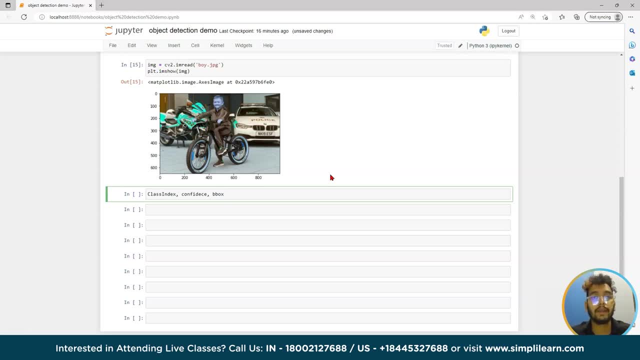 sir, new in. you found the value and I will want to update your library. so first of all I will select if my data it'll be enough for us, but first guide. I will not set that as the policy. I will not choose data. we will, doesn't, shall we? 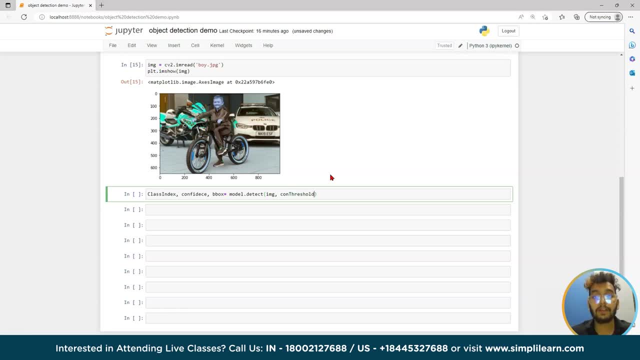 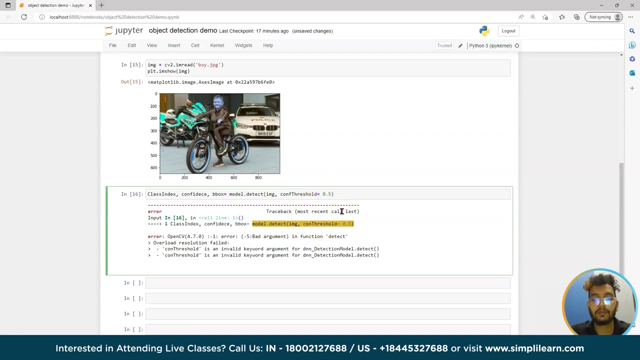 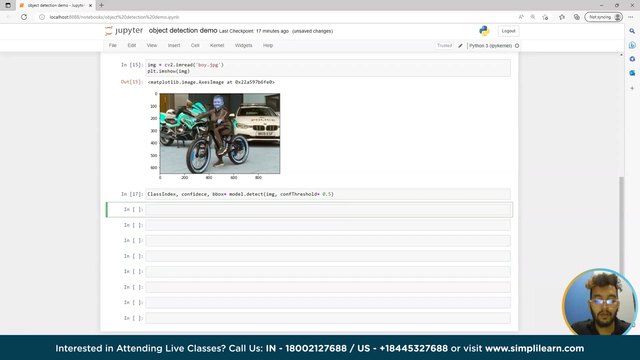 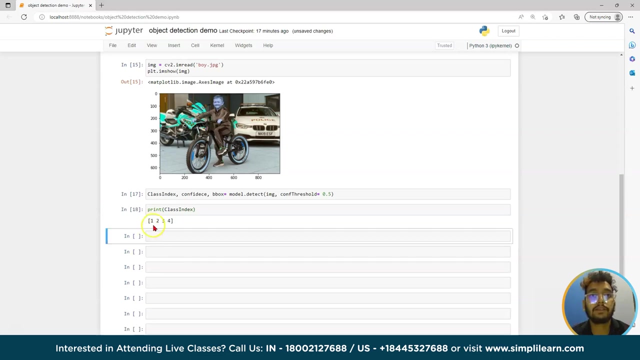 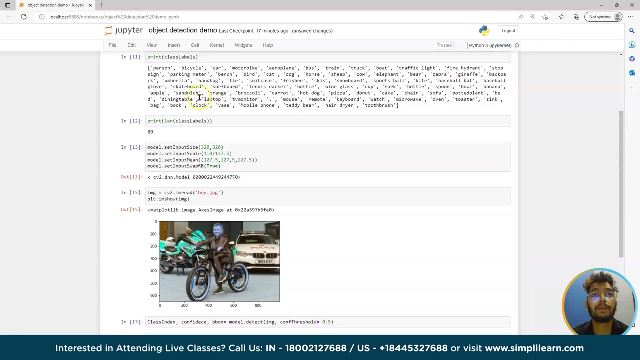 create the value. I will only" it51 competently close sign. OK, The threshold is used, for if my model will confirm it's the particular image which is the thing is correct, it will print the name. okay, let me print. and class. class index is coming: one, two, three, four. okay, so one means person, two means 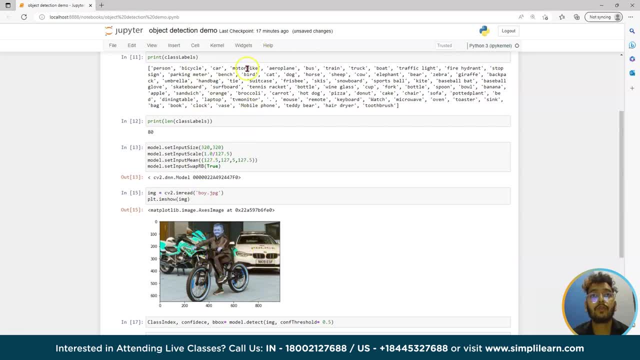 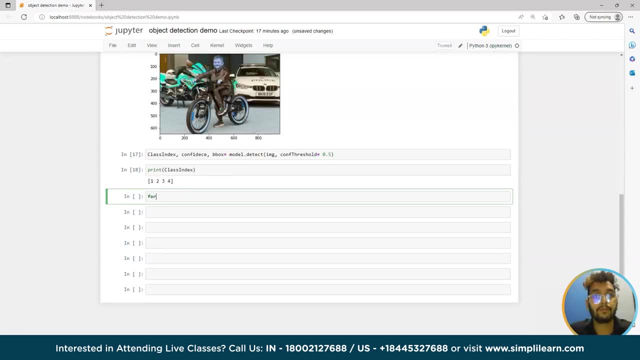 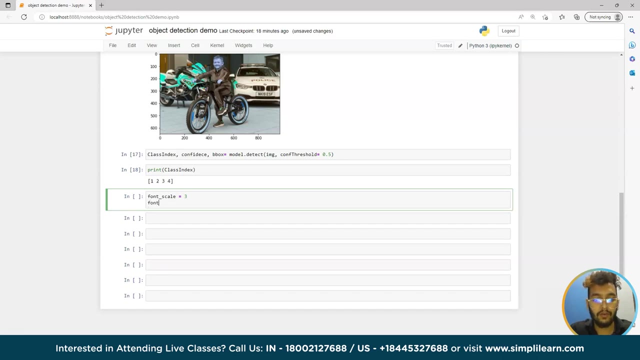 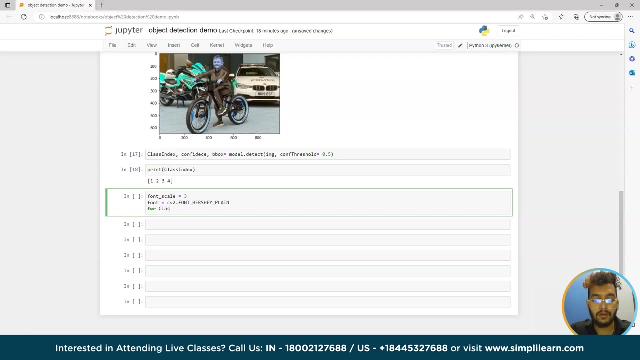 bicycle, three means car and four means motorbike. this is the class index index for particular label. I will do, I will print the boxes. font scale equals to three and the font equals to CV2 dot font, Hershey Lane or class index and the confidence and the boxes and 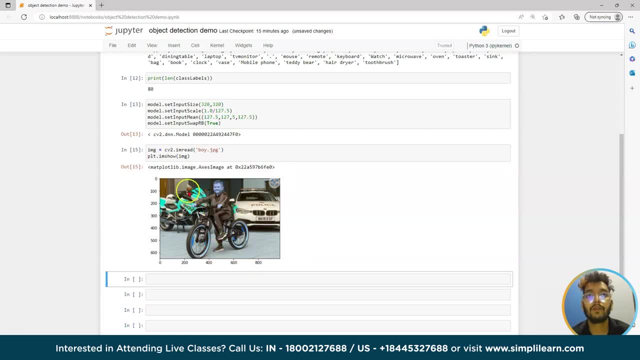 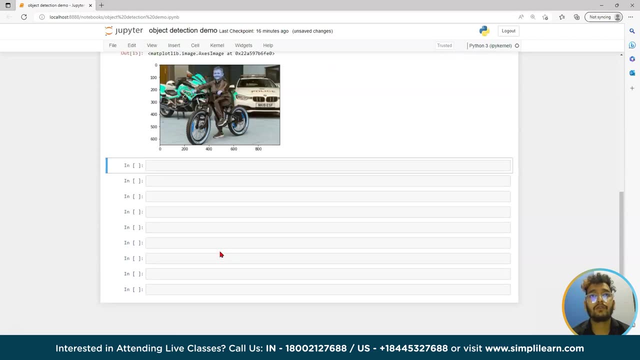 So this is the size of 320 by 320. okay, so first thing is, You can download this, the random nature from the Google. I took from Google itself. So now what we will do: We will set the class index. We will set the class index. 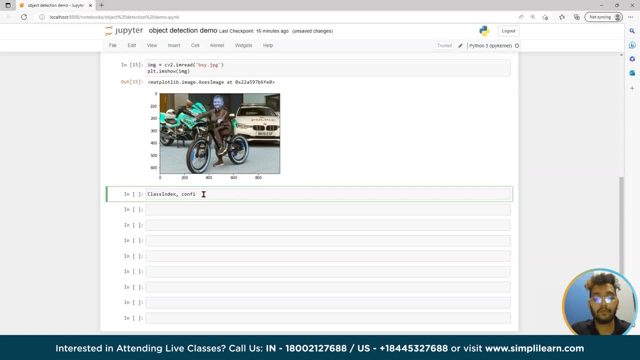 Confidence value In B box. B box is the boundary box which I will create for that particular person: cycle, motorbike and the car. okay, goes to model That you. the confidence threshold I Showed is useful. if my model will confirm It's the particular image which is the texting is correct, It will print the name okay. 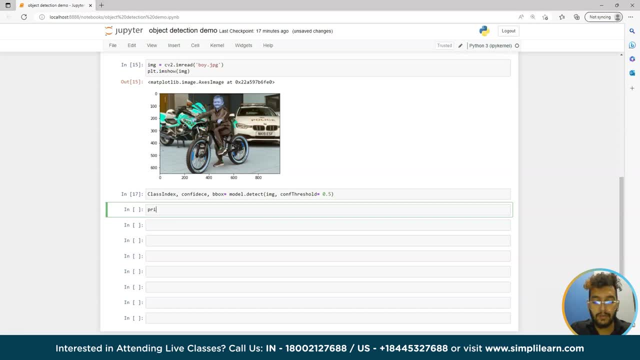 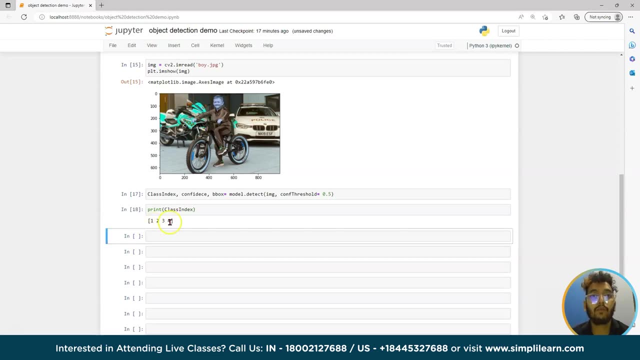 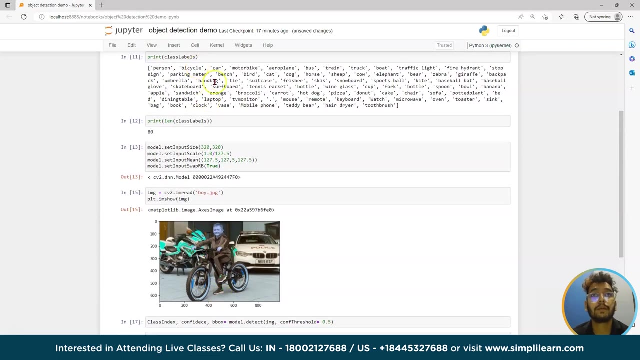 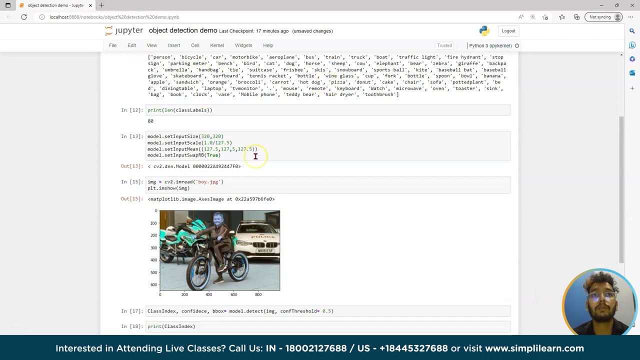 Let me print, and you, I will print the name of my model. I will print the name of my model. Class index is coming. one, two, three, four. Okay, so one means person, two means bicycle, Three means car and four means motorbike. This is the class index, index for particular level. I will do, I will print the boxes. 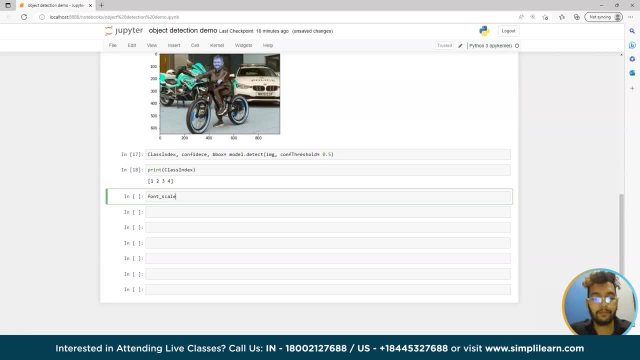 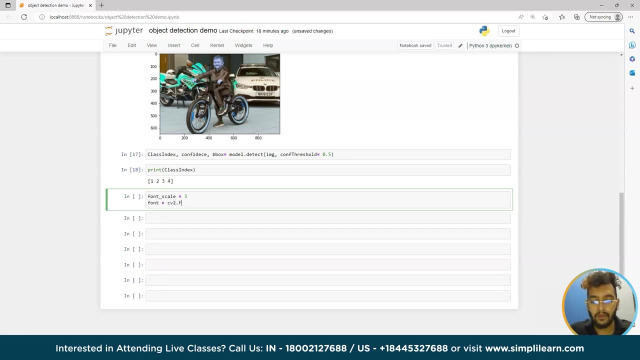 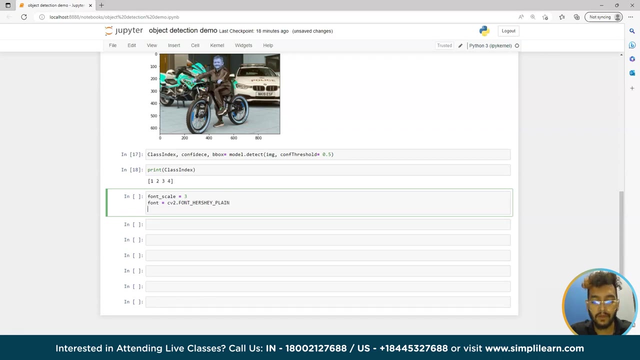 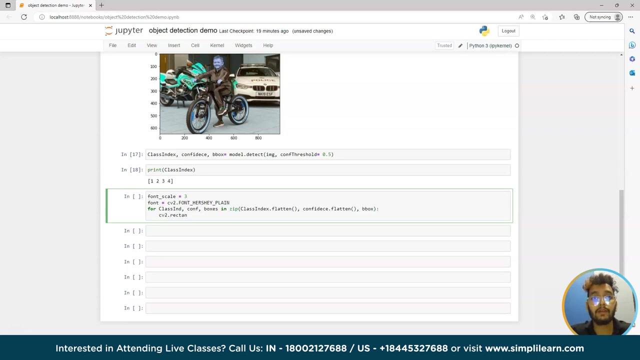 font scale equals to three and the font equals to CVT. Don't want her or class index and the confidence and the boxes and x dot pattern, confidence pattern box, the boundary box and I will write here: cv2.rectangle. make the rectangle set the image and box is: 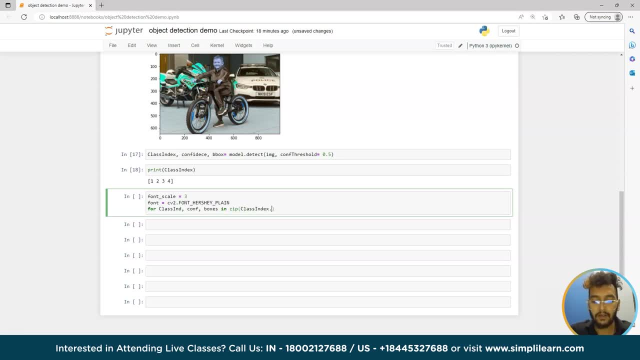 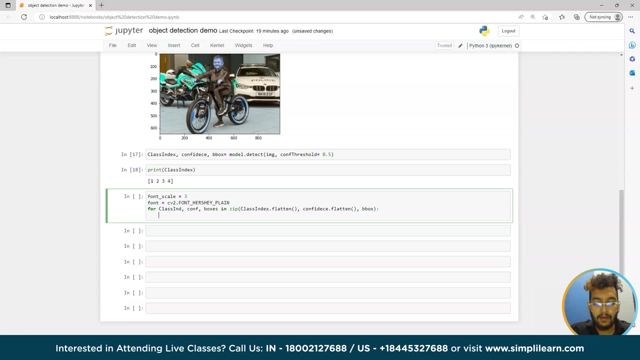 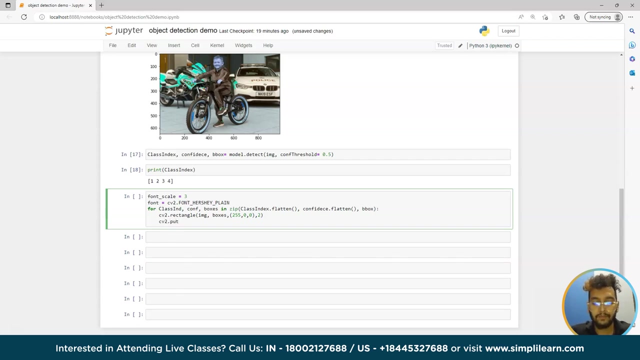 X dot atom. you, you, you, you, you. Okay, and I will write again: cb2 dot rectangle. make the rectangle that image and boxes is if comma zero, comma zero, it's the color of the box and this will be the thickness. okay, then I will write cv2 dot. put text image, then class labels. 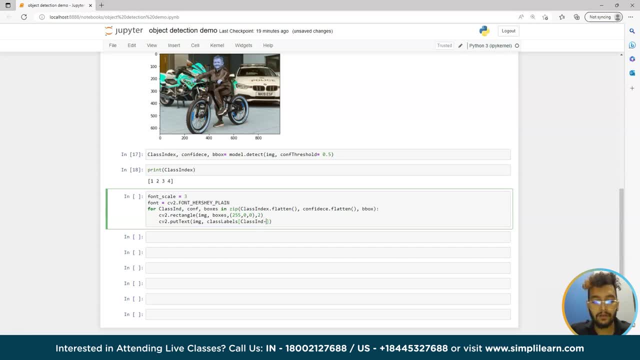 I will write class index minus 1, because always index start with zero. that's fine, and the box is 0 and boxes 1, 40, okay, scale, okay, so font scale: a color, let's do. this will be the text color: 0, 255, 0. 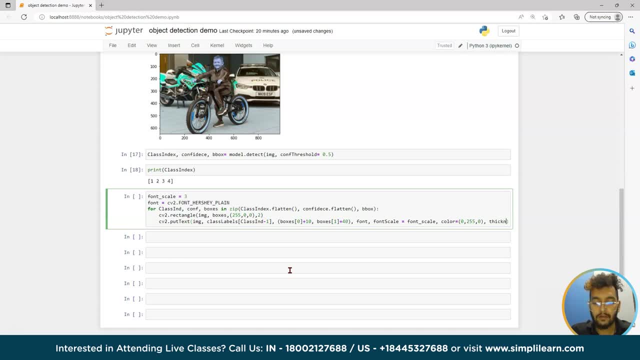 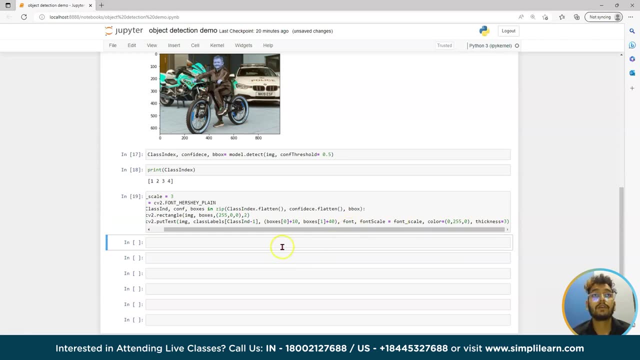 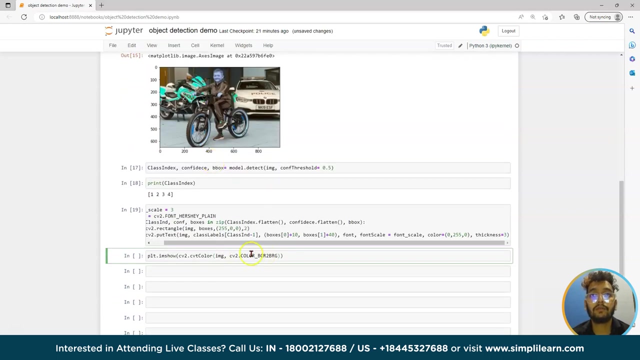 and the thickness, so three, let me run it. ah, no error. okay now plt dot, i am sure. then cv2 dot, cvt color, then comma, cv, t2 dot, color, color, then bgr to brg. that is why we wrote: swap rb equals to true, because every time we will convert bgr to brg. 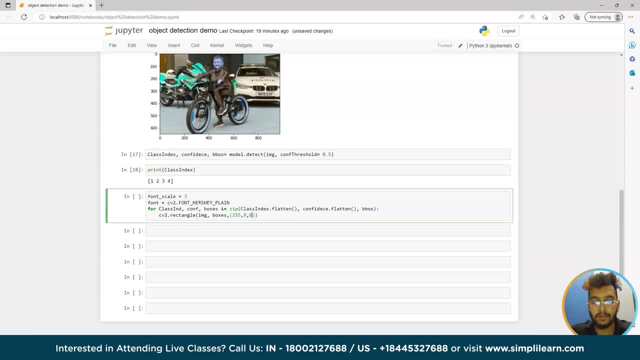 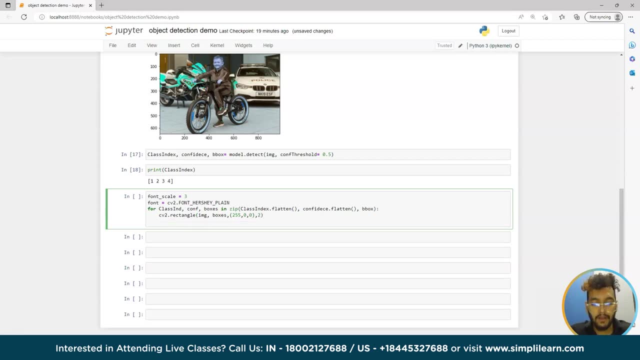 5 comma 0 comma 0. this is the color of the box and this will be the thickness. okay, then I will write cv2.put text image. class labels. I will write class index minus 1, because always index start with 0. that's fine and the box is 0. 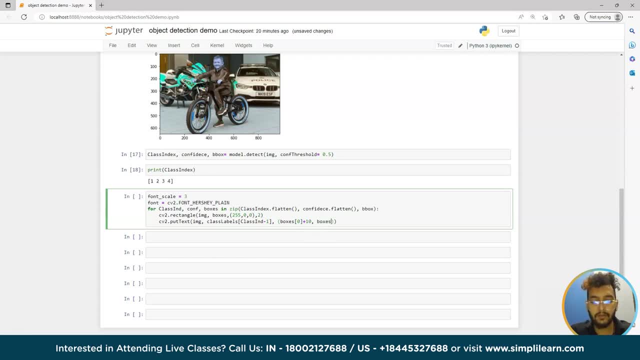 and comma boxes 1, 2, 3, 4, 5, 6, 7, 8, 9, 10, 11, 12, 13, 14, 15, 16, 17, 18, 19, 20, 21, 22, 23, 24, 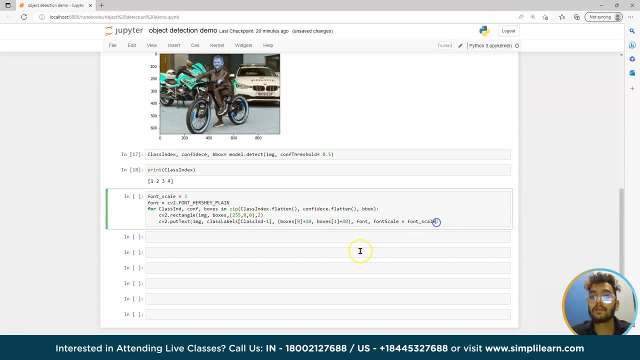 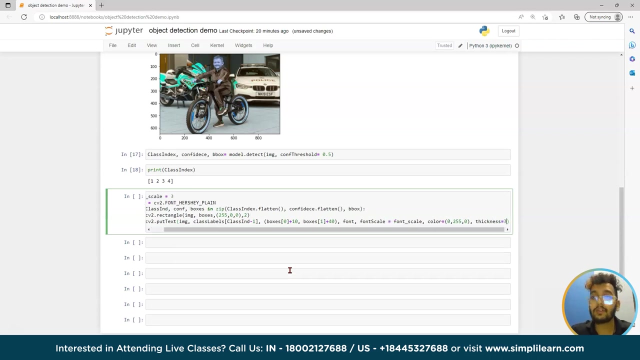 25, 26, 26, 27, 28, 29, 30, 21, 22, 23, 24, 26, 27, 28, 29, 30, 31, 32, 33, 34, 35, 36, 37, 38, 39, 40. 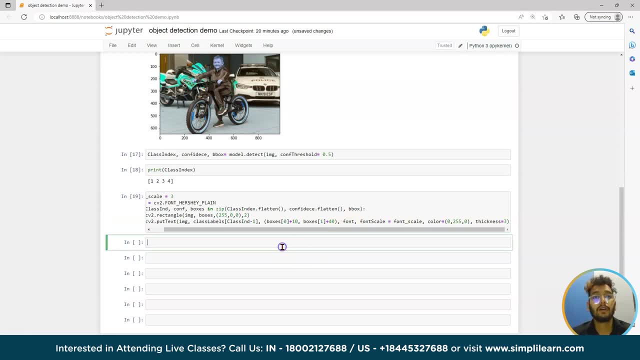 41, 42, 43, 44, 45, 46, 47, 48, 49, 50, 51, 52, 52, 53, 52, 53, 54, 55, 56, 57, 58, 59, 60, 61, 62, 63. 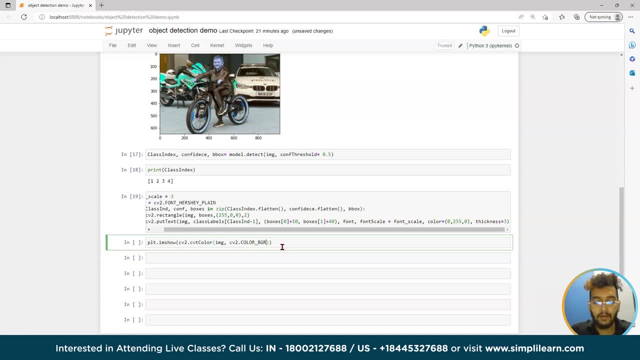 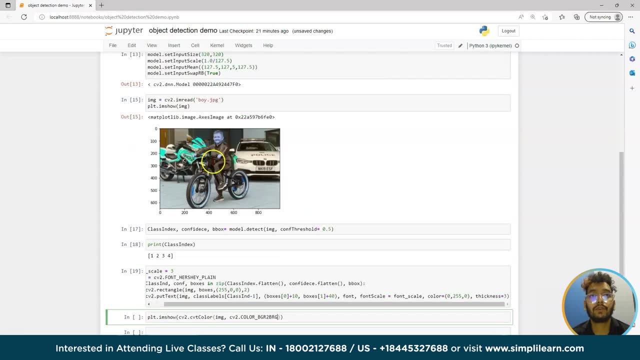 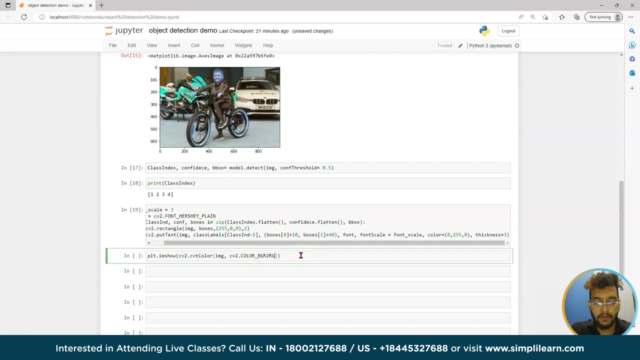 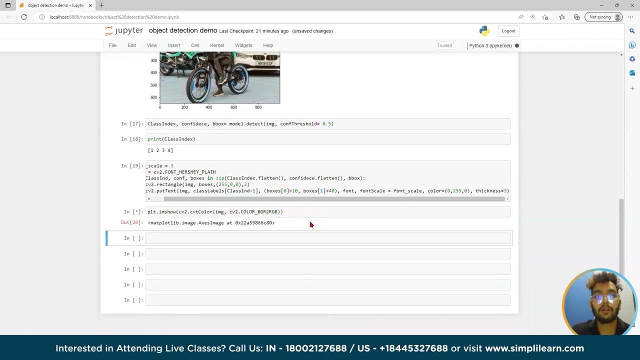 62, 63, 63, 64, 65, 67, 68, 69, 69, 70, 71, 72, 73, 72, 73, 74, 75, 76, 77, 78, 79, 80, 81, 82, 83, 84. 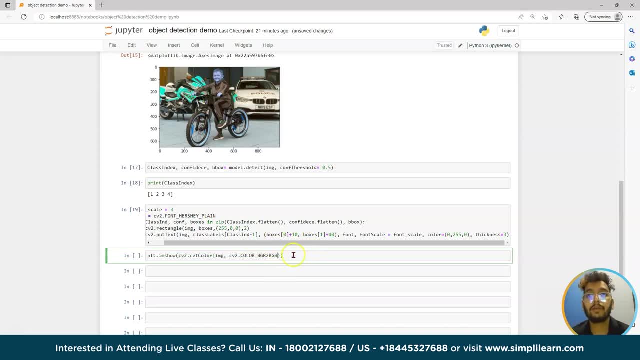 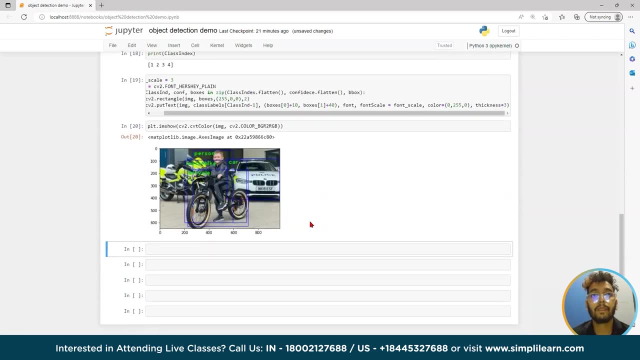 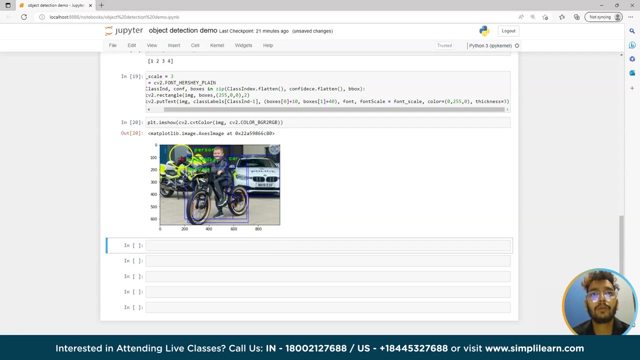 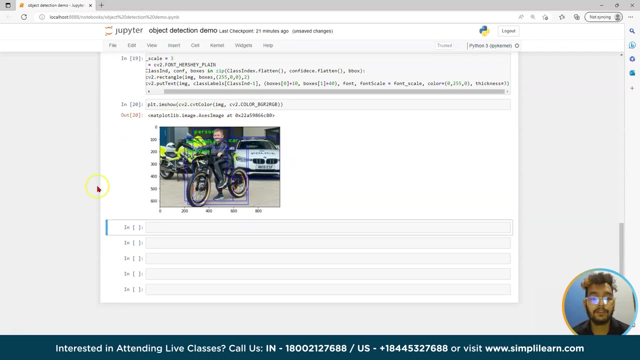 sorry, gb, rgb, so we don't have to write again and again. it will convert all the files into rgb. okay, run it. okay, as you can see, the motorbike is coming, bicycle is coming, the person is coming, the car will come, the car is coming. okay, so it's. 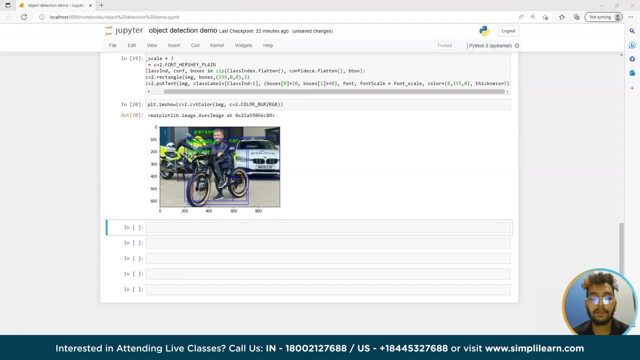 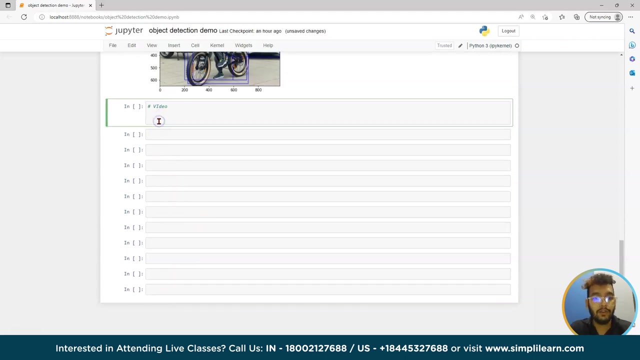 detecting the right for the image. now we will do this for the video and for the webcam. we are done with this image one and then now i will write here: okay, so this is we'll do for the video. for the video, i will write here: cap equals to capture. 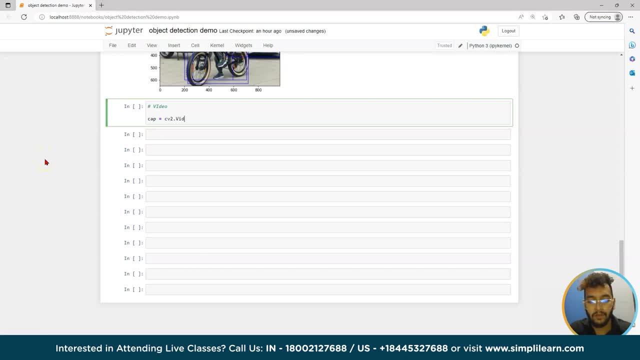 you can write any name, so cv2 dot. video capture. so you can take any random video. i took this pixels. you can take any random video. i took this pixels. click on any one by using your left or right mouse button. make sure that you press arrow and. 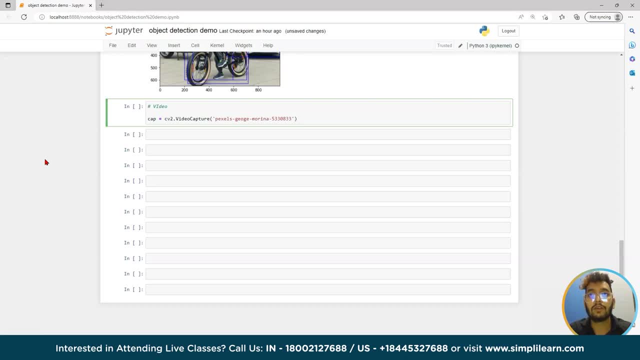 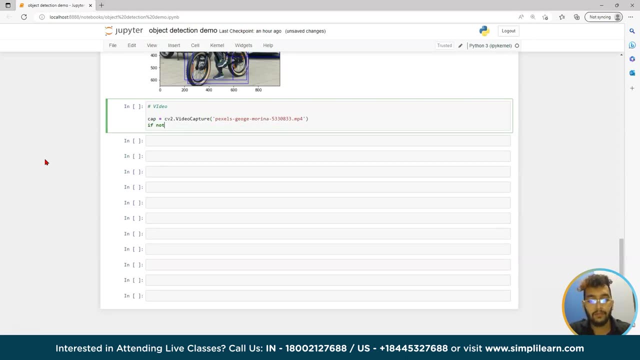 click on copyright. now you can see the image has been configured. it's untouchable, as you can see. you can click touch here. you can do the same thing like this. let me just say that. let me just make sure that you are in all the settings. 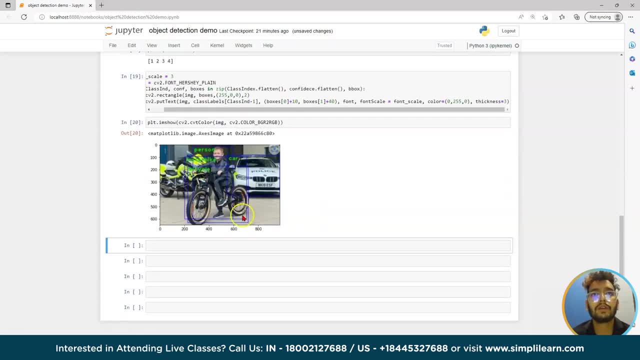 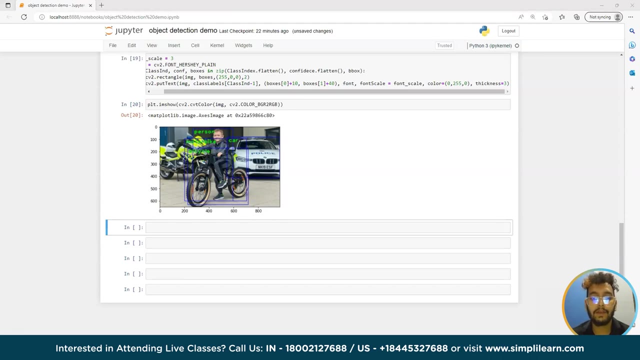 85, 86, 87, 88, 89, 90, 91, 92, 93, 93, 94, 95, 96, 97, 97, 97, 98, 98, 99, 100, 12, 13, 14, 15, 16, 17. 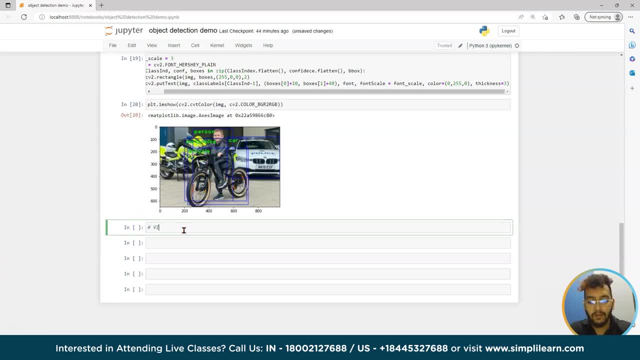 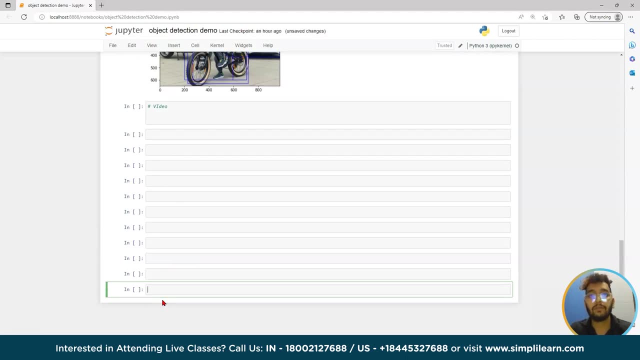 18, 19, 20, 22, 23, 24, 25, 26, 27, 28, 29, 30, 31, 32, 33, 34, 35, 36, 37, 38, 39, 40, 39, 40, 41, 42. 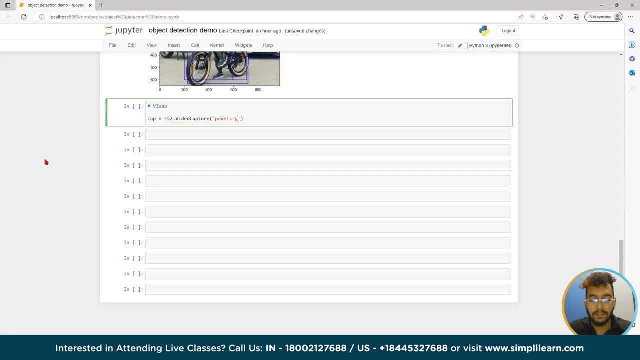 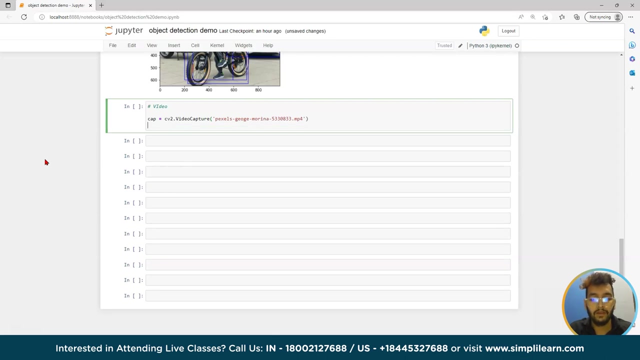 43, 44, 45, 46, 47, 48, 49, 49, 50, 51, 52, 53, 53, 54, 55, 56, 57, 68, 68, 69, 69, 70, 71, 72, 72, 73. 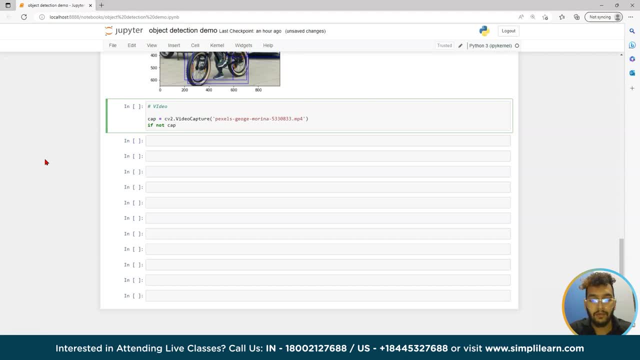 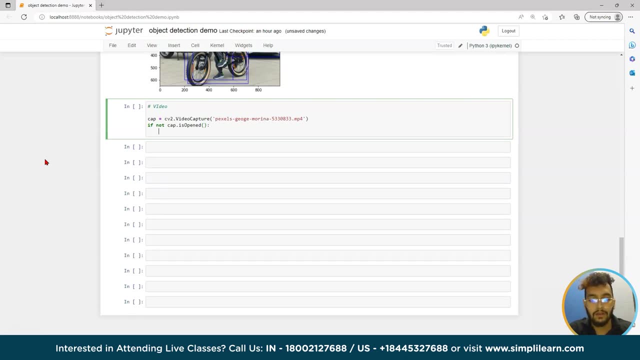 74, 75, 76, 77, 78, 78, 79, 80, 81, 82, 83, 84, 85, 86, 87, 88, 89, 90, 92, 93, 93, 94, 95, 96, 97, 97. 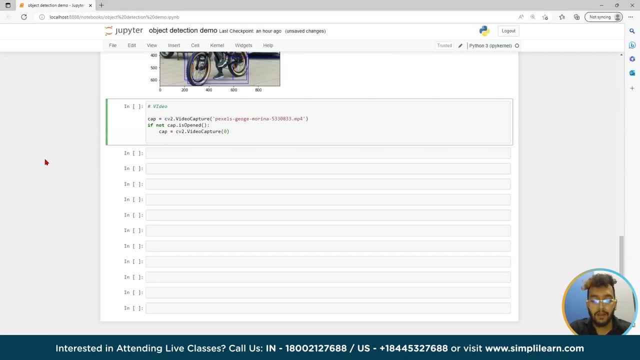 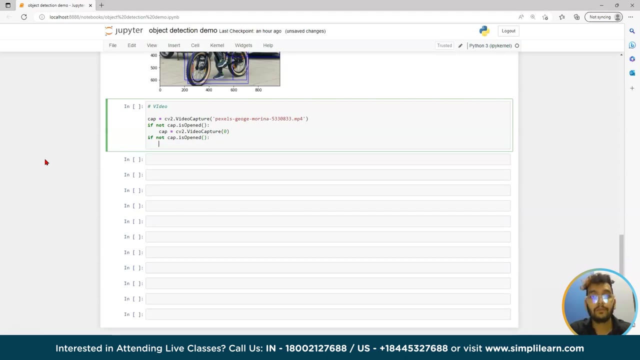 98, 99, 100, 100, 100, 13, 24, 25, 26, 27, 38, 39, 39, 40, 41, 42, 43, 44, 45, 46, 47, 49, 50, 51, 52, 53. 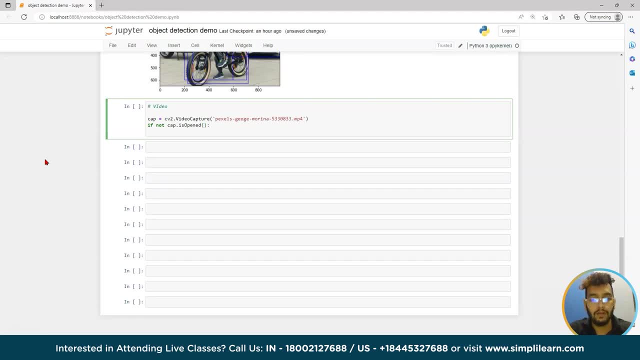 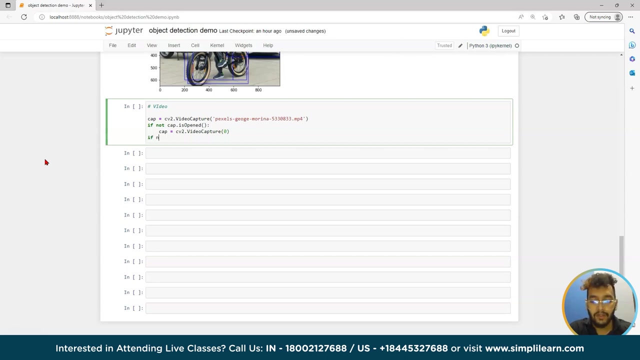 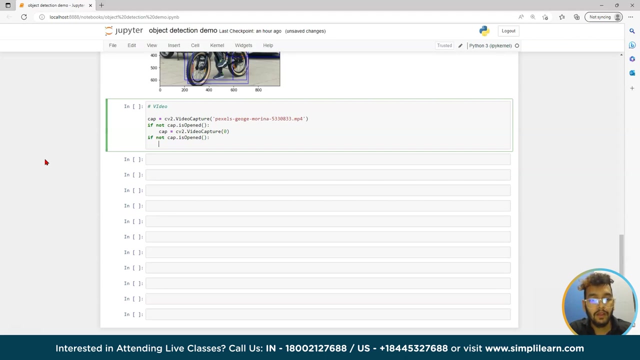 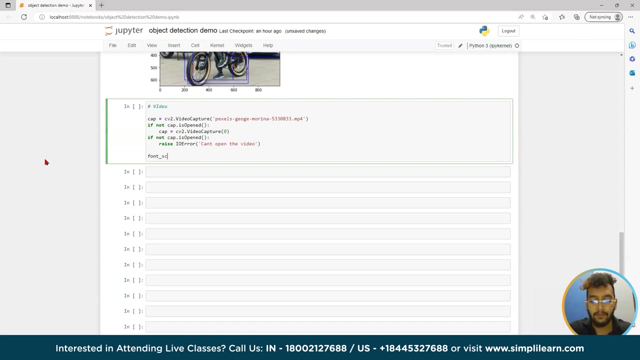 causes that. you can see that this is what you are seeing over here. I will write: cap equals to cv2. sorry, cv2 dot video capture 0 and if not, cap dot is open, then then raise output error and open the video. and open the video here. everything will be the same. font scale equals to 3. okay, font equals to cv2. 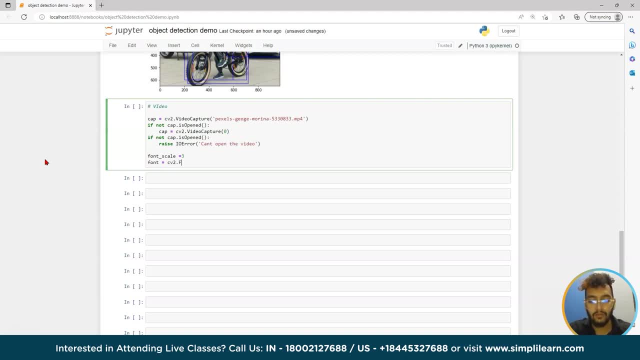 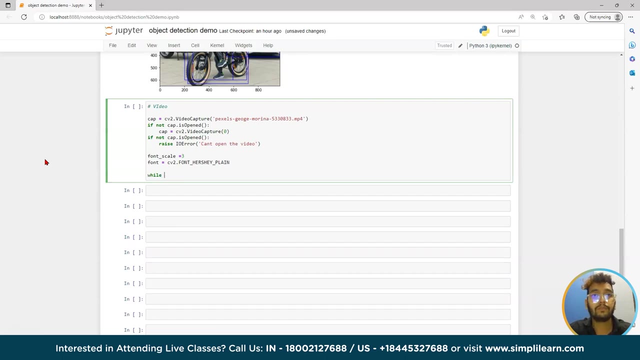 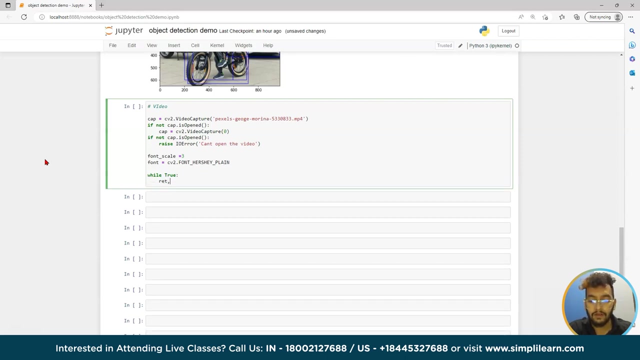 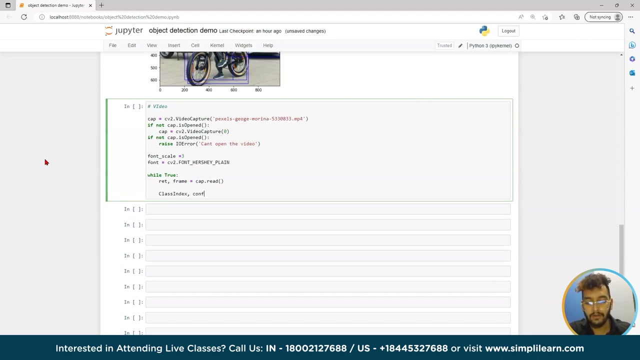 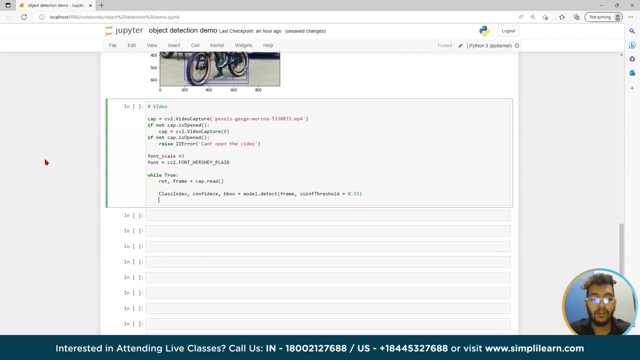 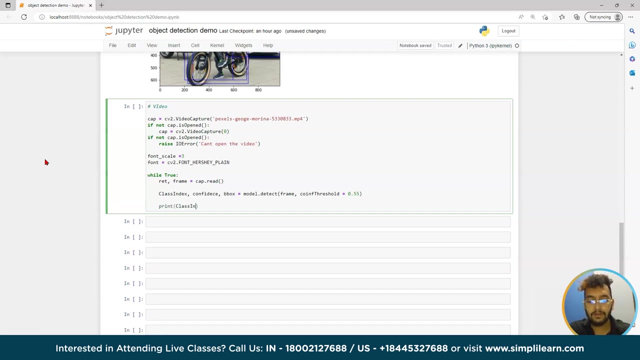 dot font harshae in. okay, so here I will write: while true from a frame was to cap dot sheet, this for the reading of the file, the same I will write: class, index, comma, confidence. my boundary box was to model dot- detect him, and the confidence threshold so 0.55. okay, everything is the same we did before. I have's print last index, okay. 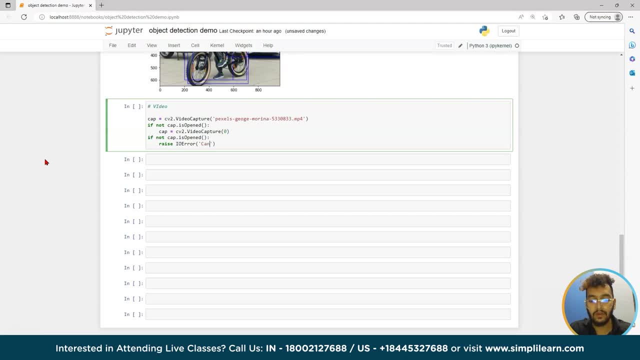 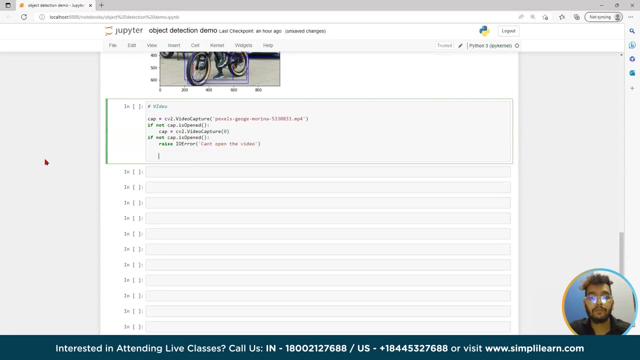 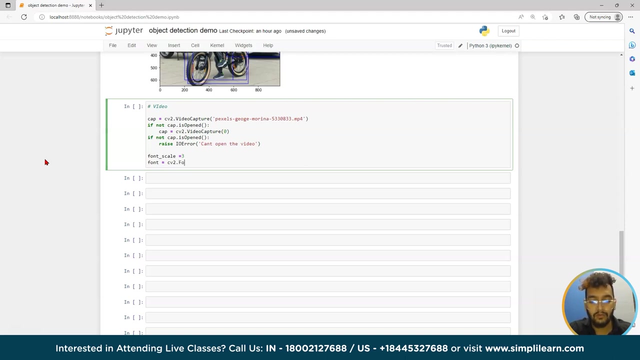 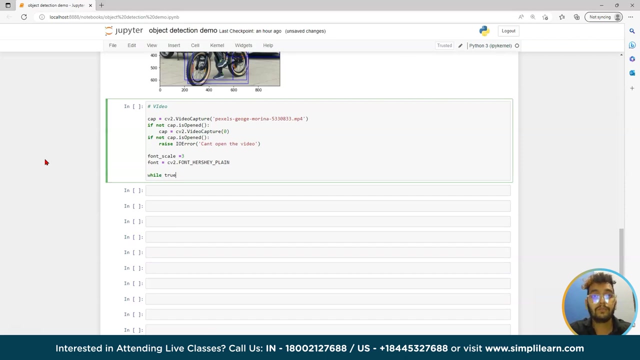 53, 53, 54, 53, 54, 55, 66, 67 the video and open the video here. everything will be the same. font scale equals to 3. okay, font equals to cv2.font-harshain. okay, so here I will write while true. 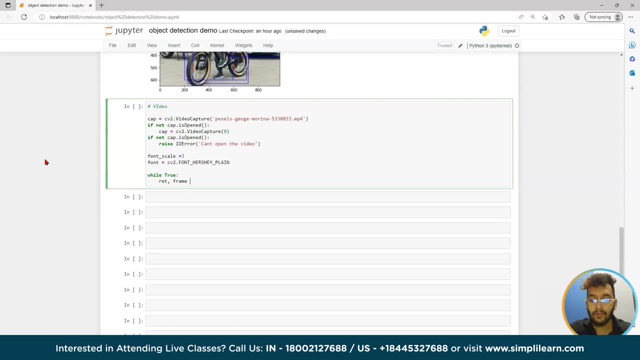 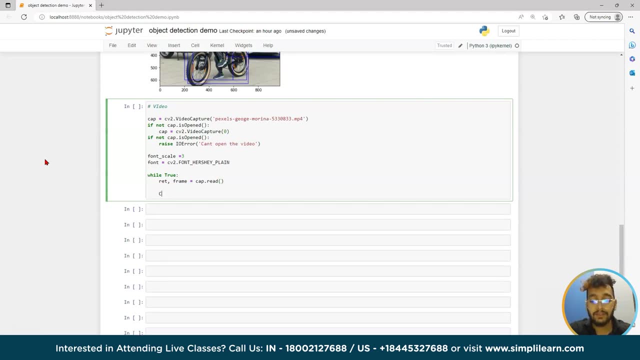 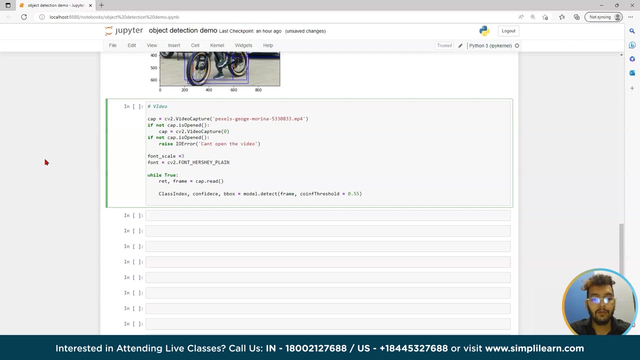 I'm a frame was to cap dot sheet. this for the reading of the file, the same I will write: class, index, comma, confidence. my boundary box was to model dot, detect him and the confident threshold was to 0.55. okay, everything is the same we did before, so here I will print class: 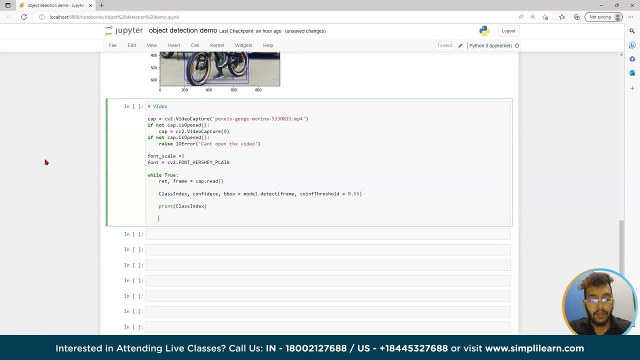 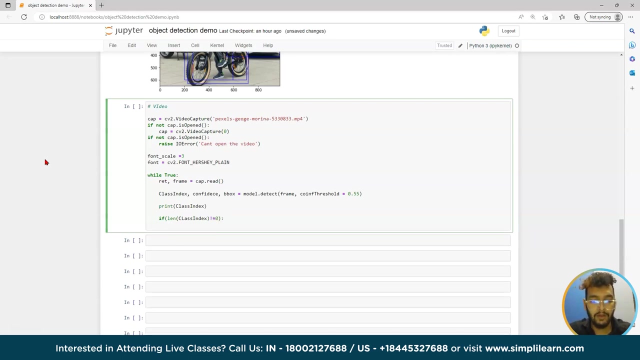 index. okay, so here I will write if and the class index that's not equals to 0, and what to perform is here after at 4: class index comma, confidence comma. boxes in zip us X dot. flattened. flatten is The Lairs. okay, go on, produce flatten. 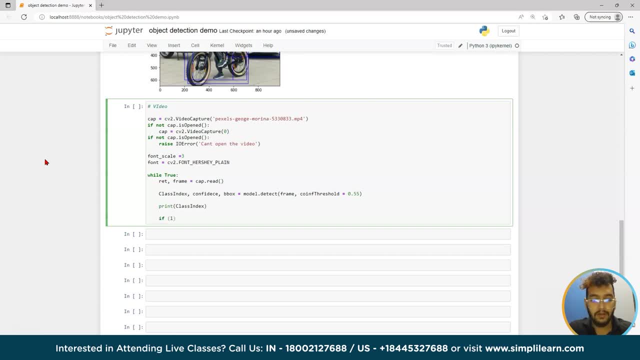 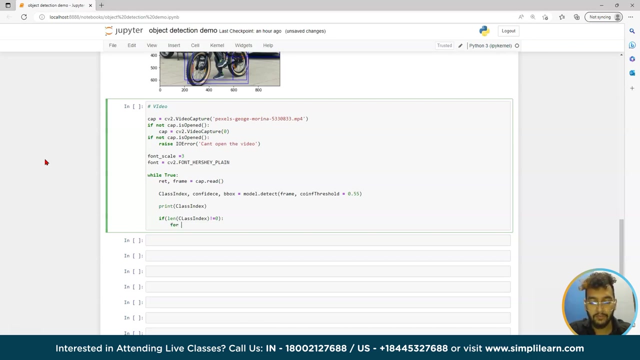 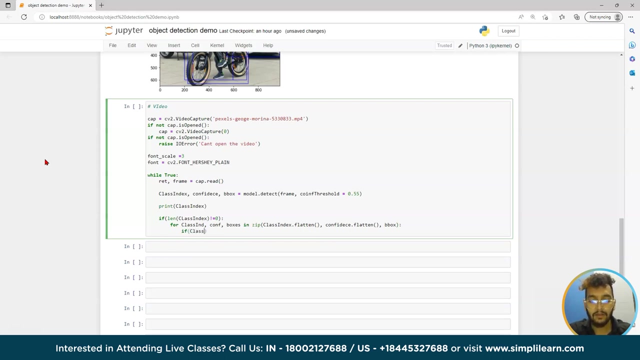 so here I will write: if and the class index does not equal to 0, then what to perform is here. I have to add for class index comma, confidence comma boxes in zip: class index dot flatten, flatten is a layers okay, confidence dot flatten box. and if class index is greater than equals to 80. and what to do then I will copy from: 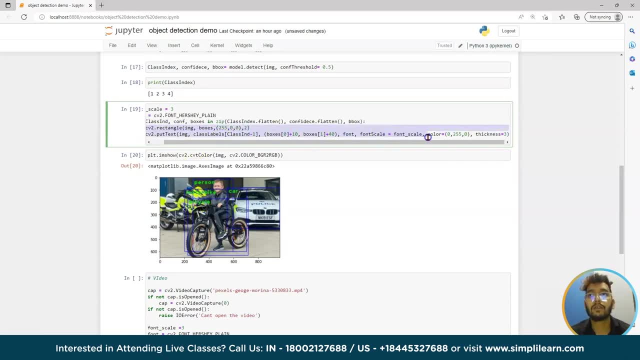 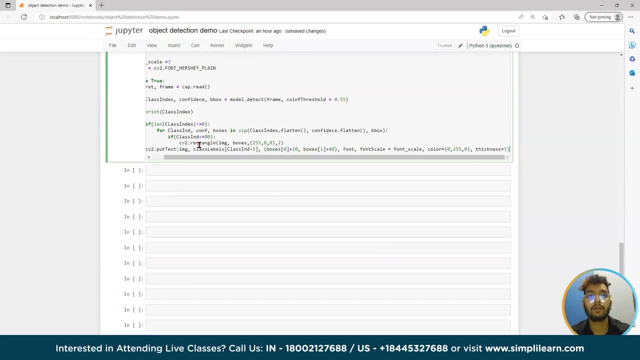 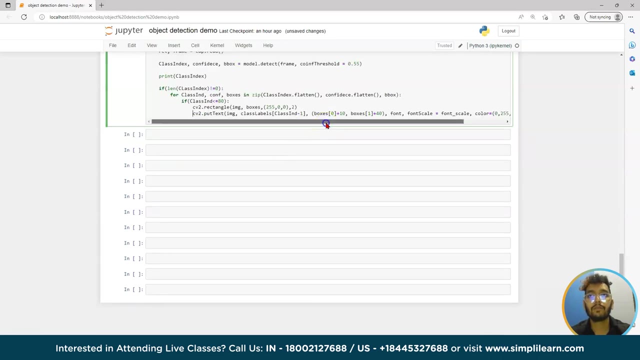 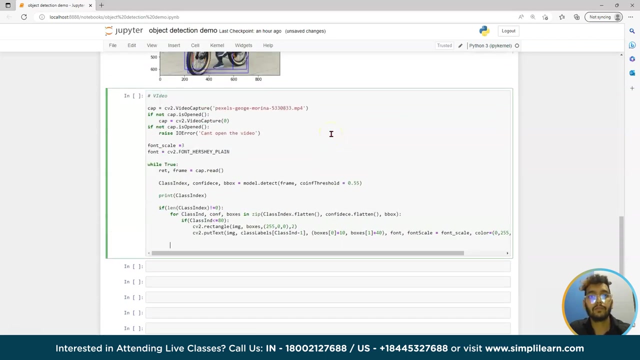 here. Okay, the same thing I have to write here. here I will write cv2 dot. I am sure this will be the return in the frame: object detection: Okay, By simply learn and frame, If cv2 dot wait key two and zero ffx equals to oi dot wait key two and zero ffx equals. 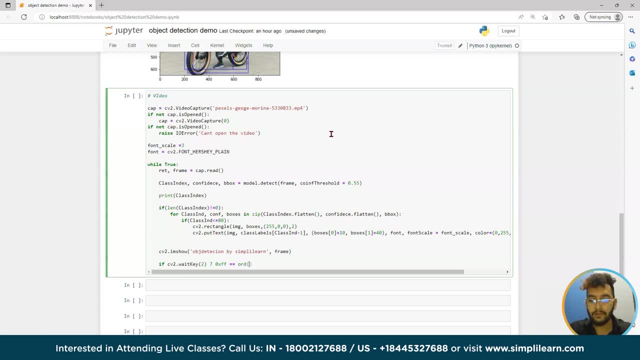 to oi dot wait key. Okay, Okay, If cv2 dot wait key two and zero fx equals to oi dot wait key two and zero fx equals to oi dot wait key, Okay, Then then I will write break- Will you break when? and get into two. the wait key will be two. 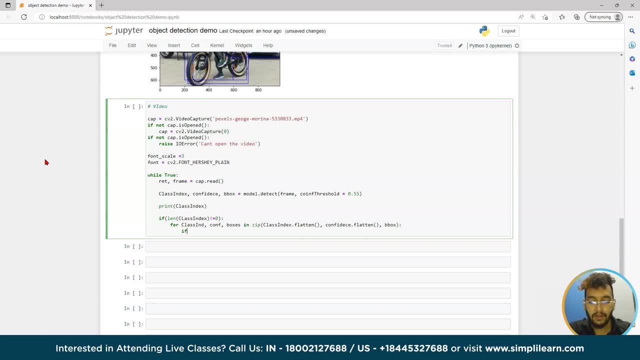 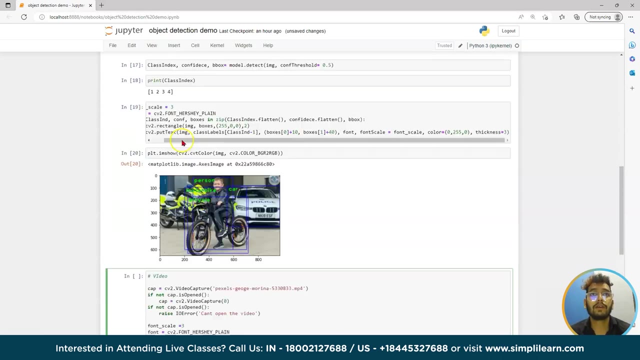 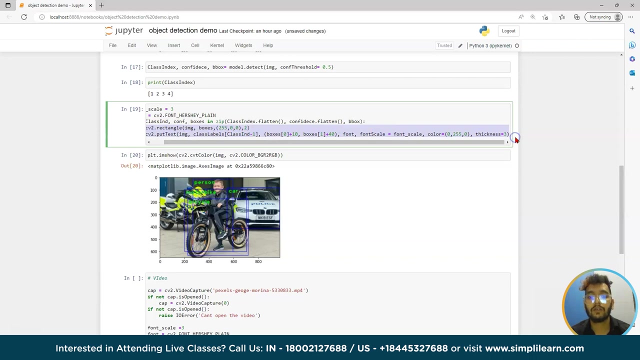 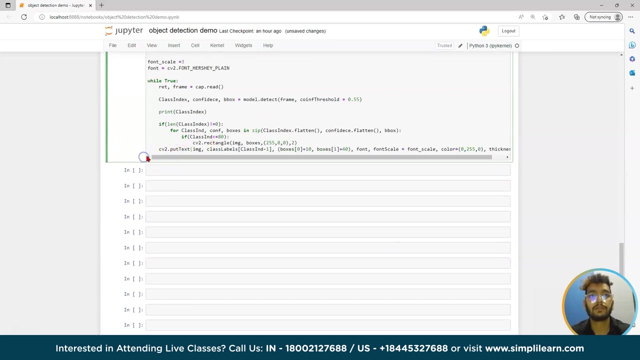 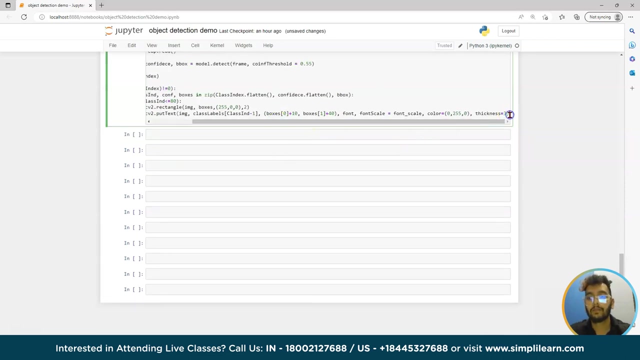 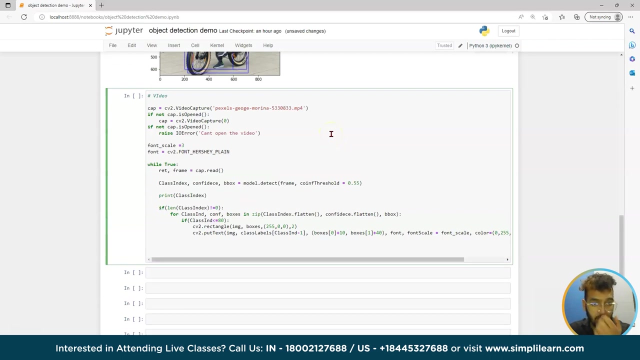 you box and if class index is greater than equals to 80, and what to do, Then I will copy from here the same thing I have to write here. So here I will write cv2.. I am sure this will be written in the frame. object detection by simply learn and frame. 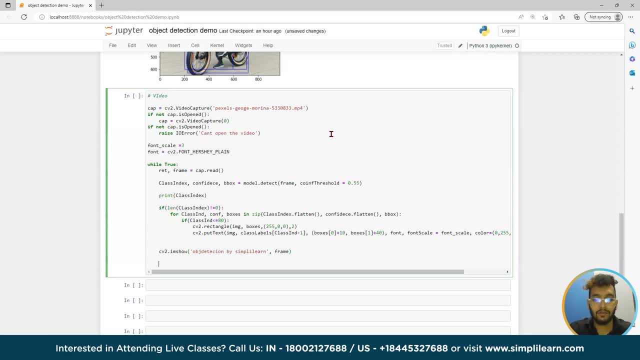 So if cv2.. Weight key 2 and 0, ffx equals to ordq, okay, Then here I will write break. Will you break when gradient to 2.. The weight key will be 2.. Okay, I will tell you what is the weight key. 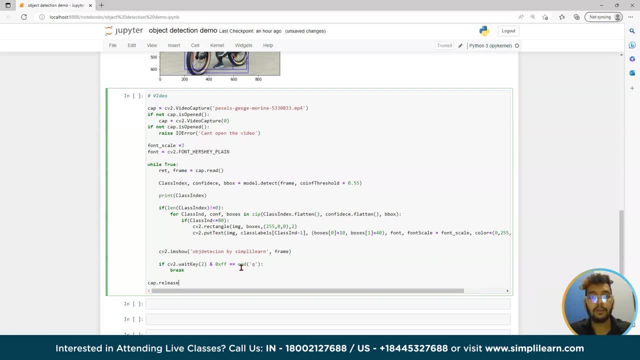 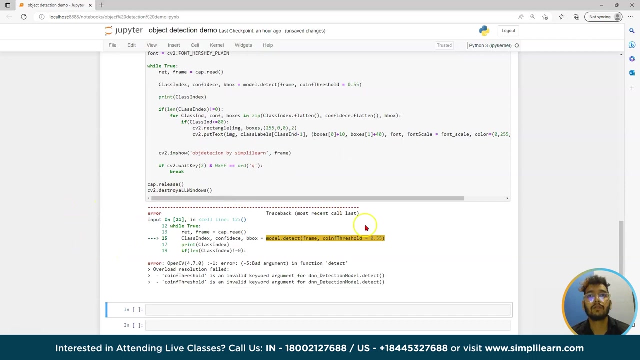 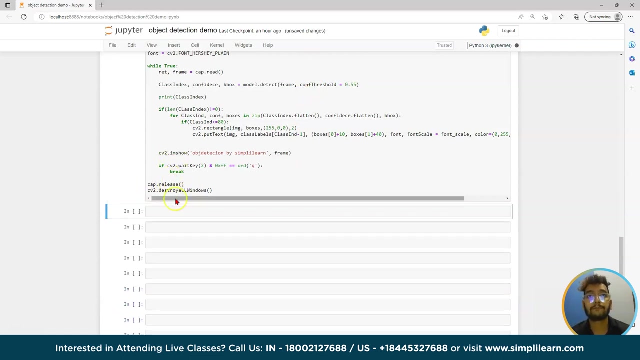 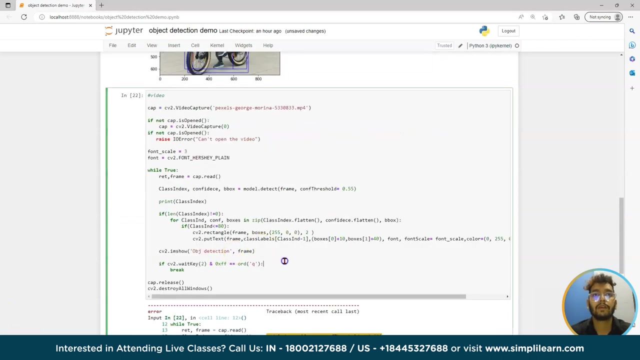 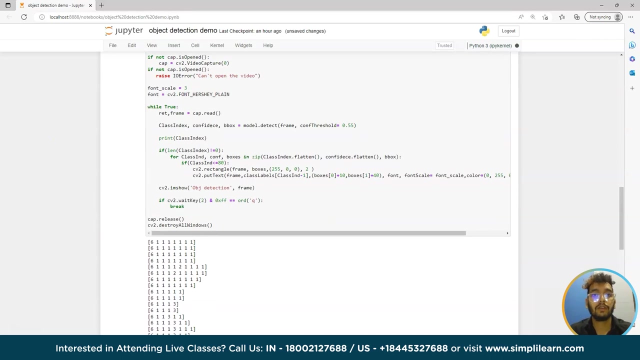 Here I will write: caprelease and cv2.destroyAllWindows. okay, So now let me run. Let's see here There will be a error. okay, cvPythonProgrammingLanguageModules. Let me run it again. The weight keys- okay. 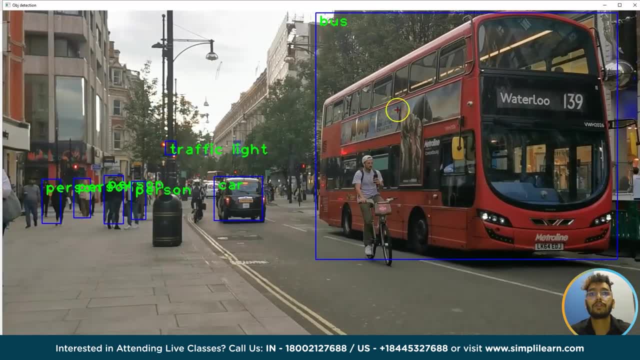 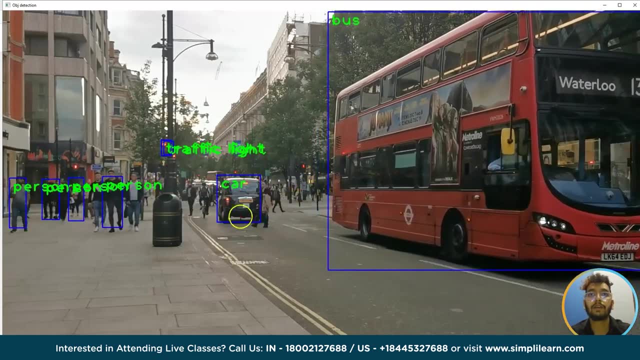 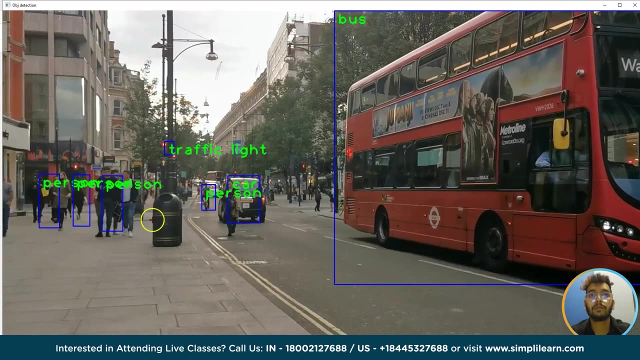 So the video is here. The video is here. As you can see, it's the bicycle, the person, the person, the bus, car, traffic light, the person, person. So our object detection for the video is coming right, okay. 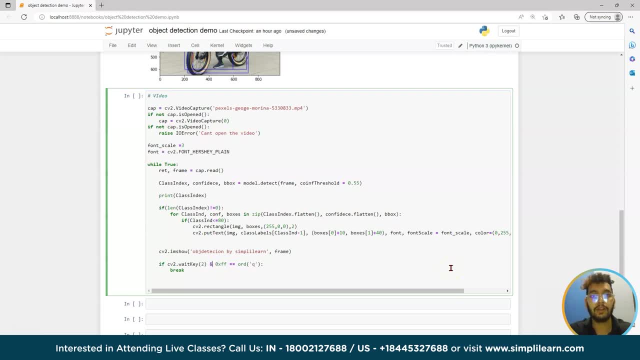 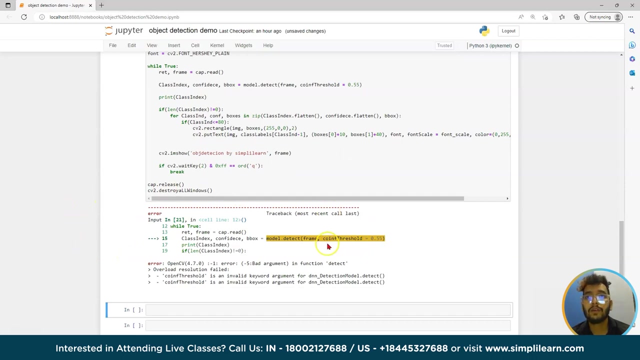 Okay, I will tell you what is the wait key here. I will write cap dot release and cv2 dot break. Okay, I will get into two, Okay, No, No, destroy all windows. okay, so now let me run. it's here, okay. 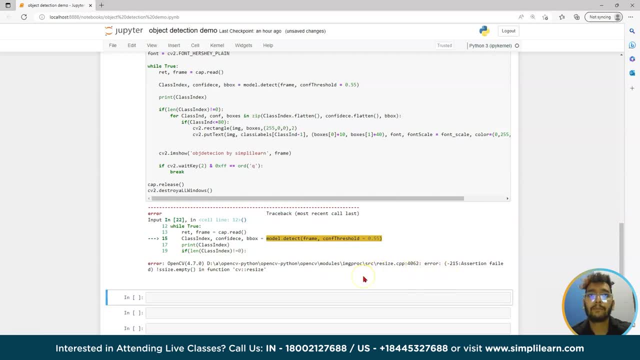 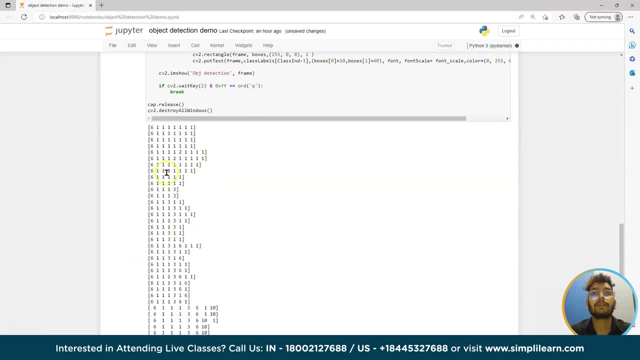 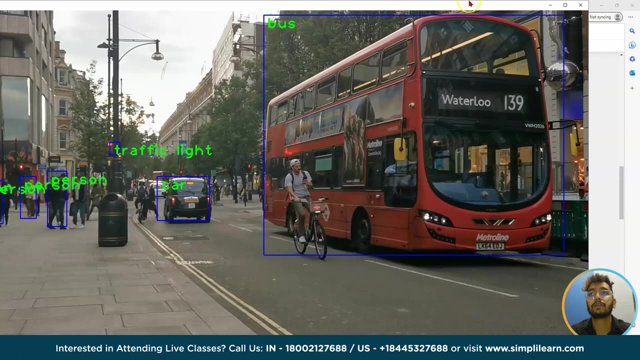 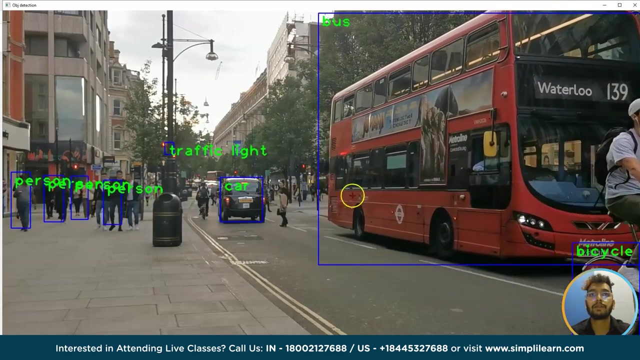 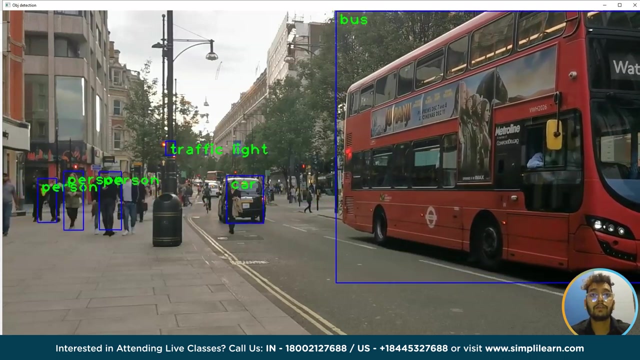 you, we don't eat again the veggies. okay, video is here. the video is here, as you can see. see: bicycle the person, the personal, bus, car, traffic light- the person, person. so our objective action for the video is coming right. okay, person, okay, person the person. we done it again. give a cities an article. now, here we just His. 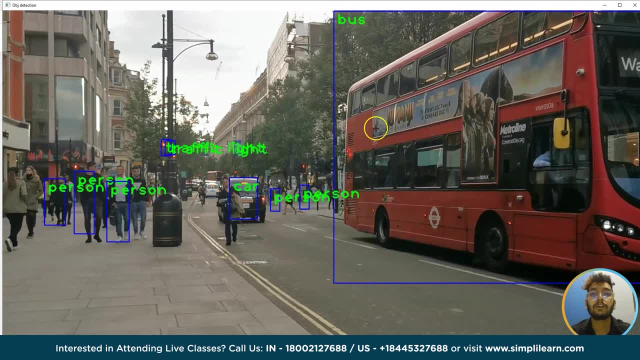 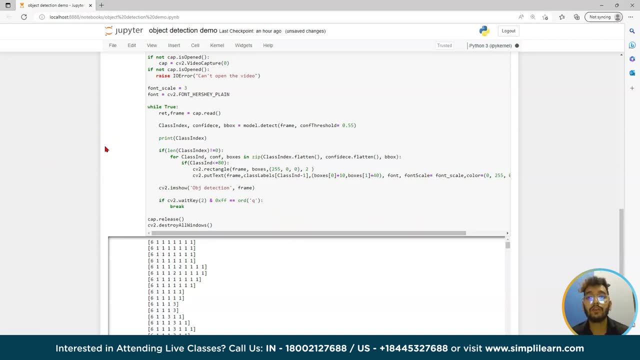 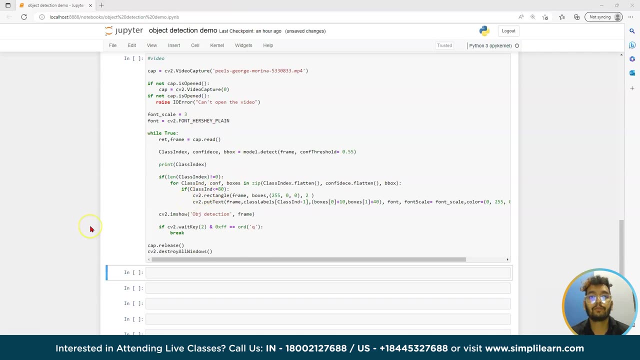 wave the person, say, as you mentionedauen minutes to the person, at least on our sister epic light. but this is how you can do for the video. okay, now, let's, we will do for the webcam live. so this is for the video. so if you want to do for the, 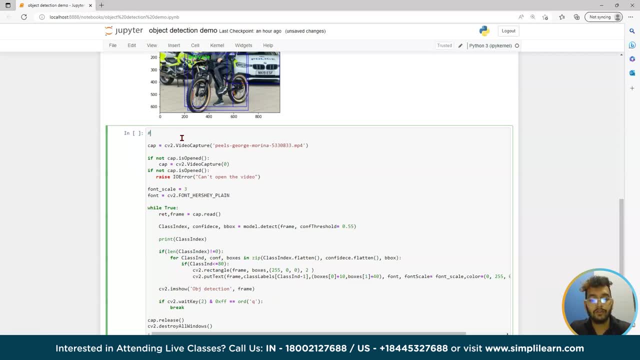 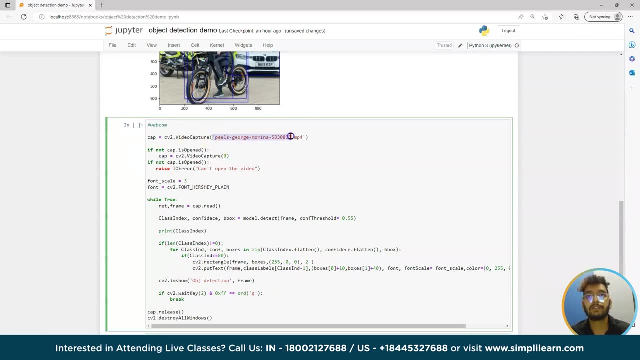 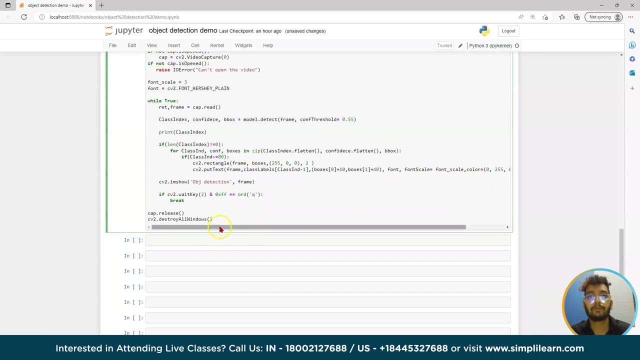 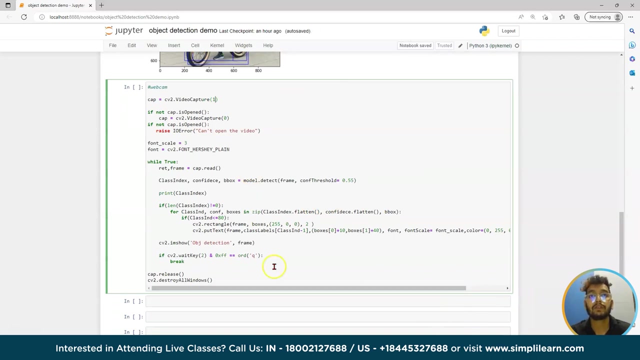 webcam with. okay, so we need to just change one, one thing only we have to change. instead of giving the file, we have to write one here. okay, the rest will be the same what it so I have to just shut down my webcam. so let me shut down the webcam and get back to you. 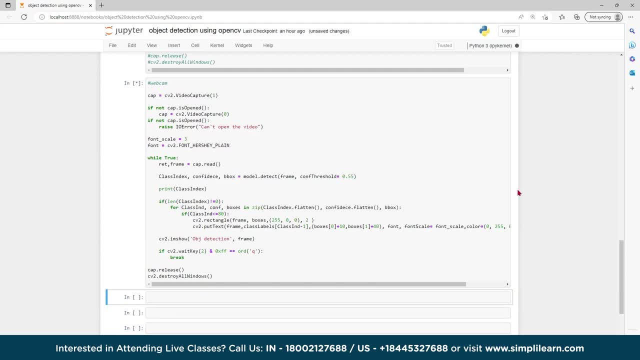 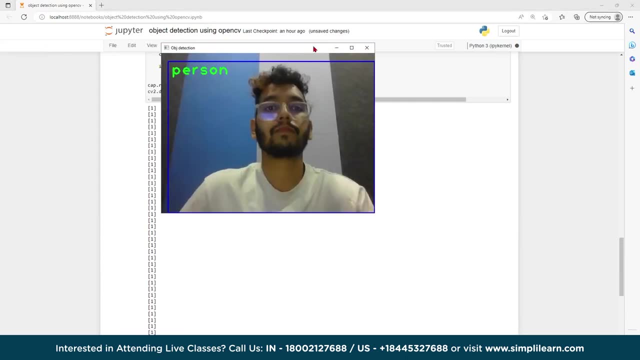 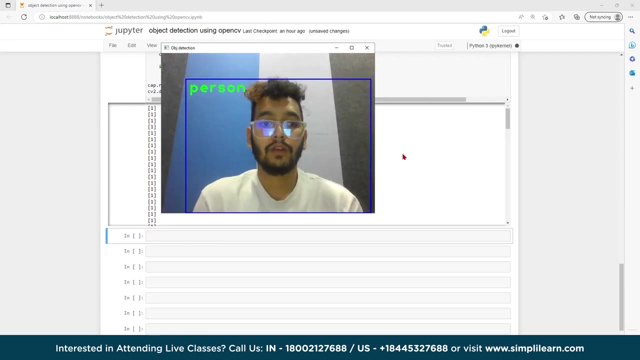 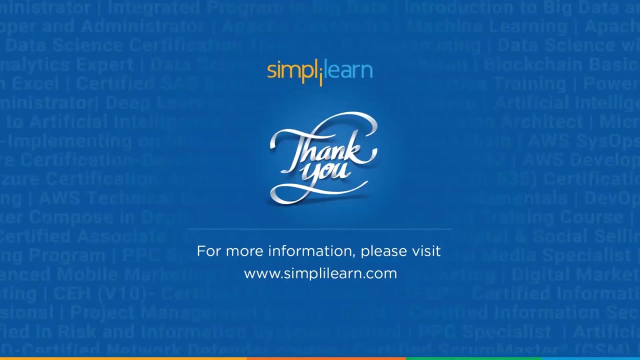 deputy you. so this is coming right. okay, so I, if I will show this, the mobile phone is coming right now. okay, so this is how you can do the correct object detection. okay, so, okay, nee. So if you enjoyed this video and if you want this full code how to do so, you can comment.